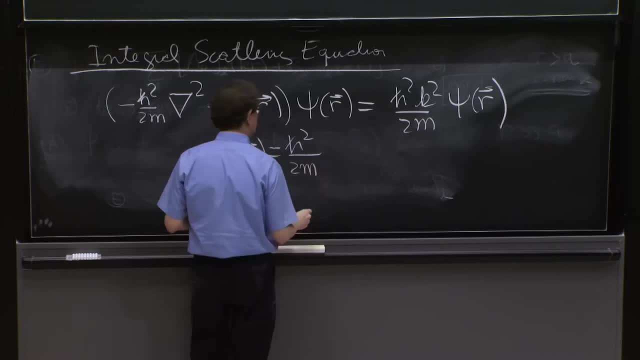 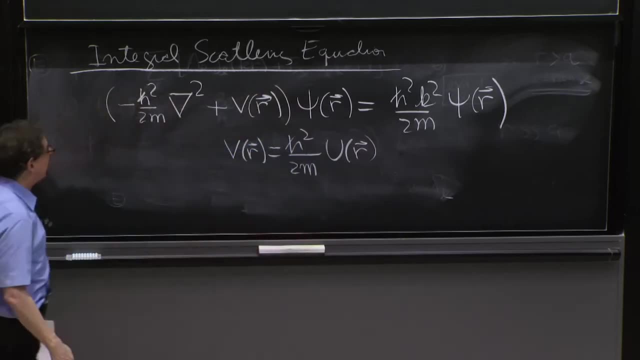 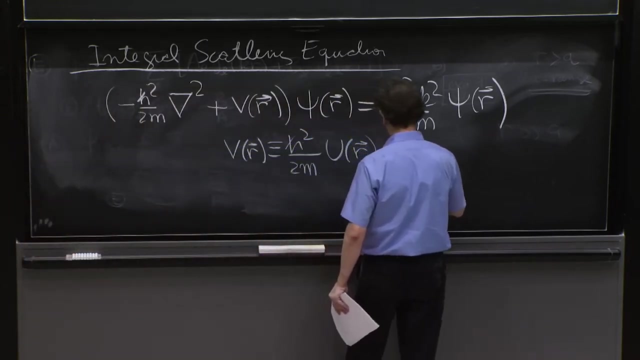 And I'm going to do that by multiplying over 2m. u of r? u still reminds you of a potential, I think, And it's a good thing. It's a definition of u of r. It's a definition, And in that way I can get rid of the h bars. 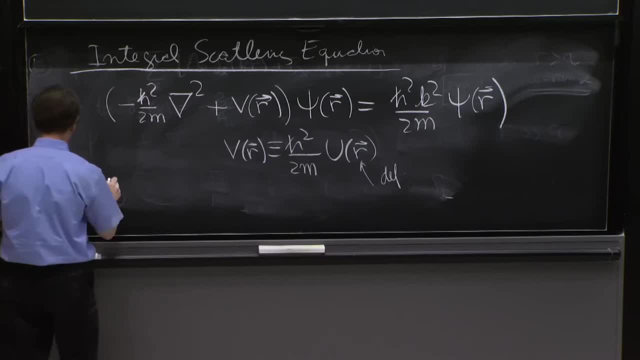 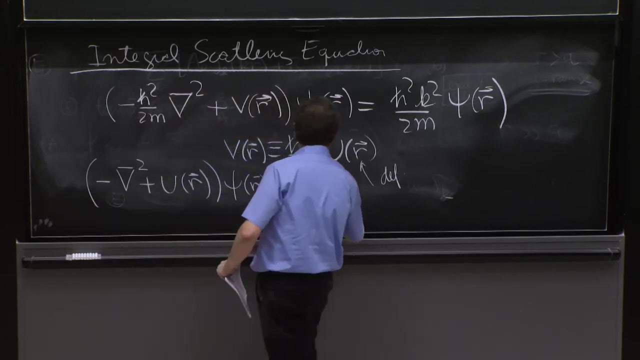 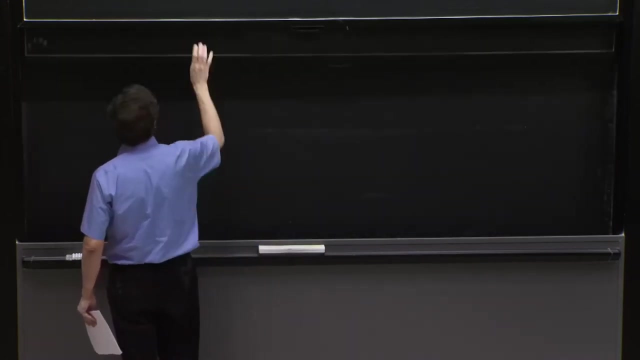 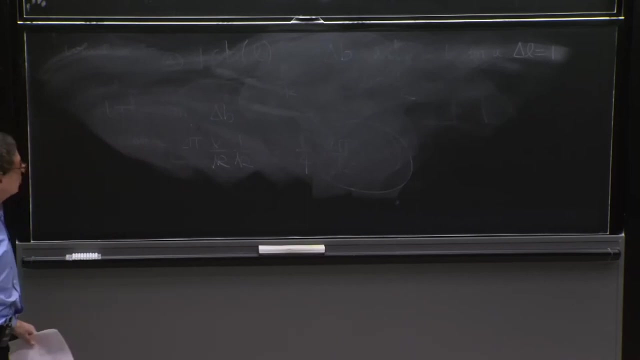 in the Schrodinger equation. And what do we get? We get minus. We get minus u of r from Laplacian plus u of r. acting on psi of r is equal to k squared acting on psi of r. OK, That looks nice. 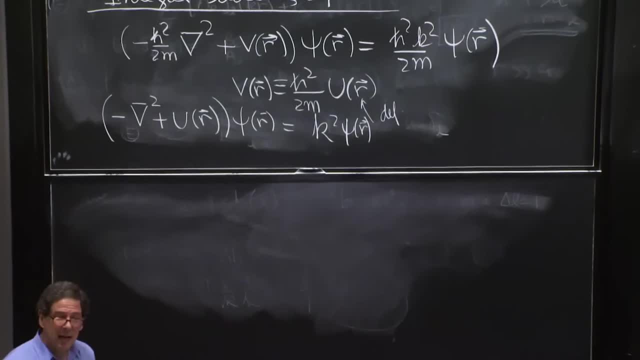 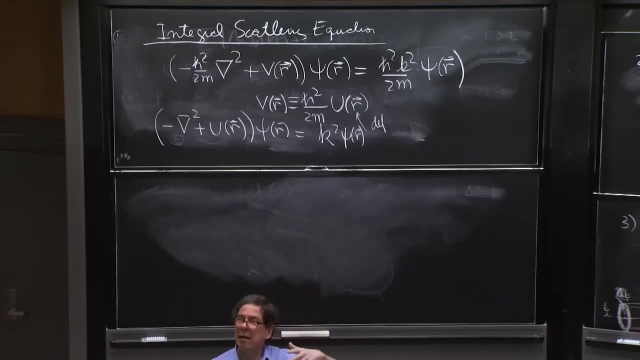 So So what I'm going to do is I'm going to do a simple operator, if you put it in a way that the left-hand side is kind of a nice simple operator And the right-hand side involves a potential. So I'll move it along so that I can pass the nabla squared. 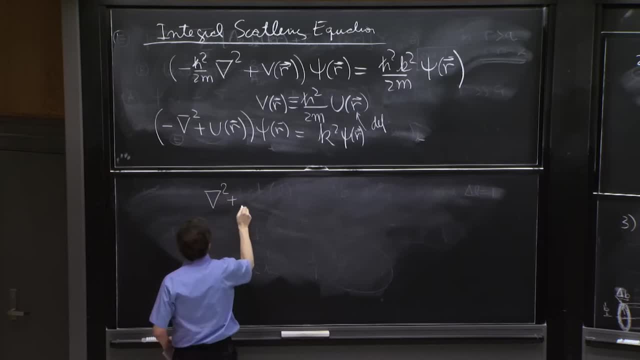 to the right, but then make that the left-hand side. So this will be Laplacian squared plus k squared on psi of r, And the left-hand side is equal to u of r, psi of r. OK, So we've written, we've done nothing so far. 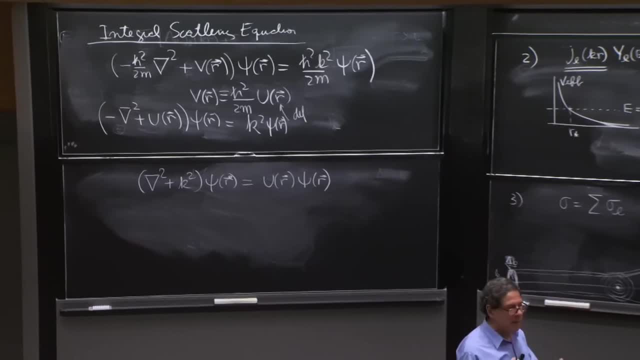 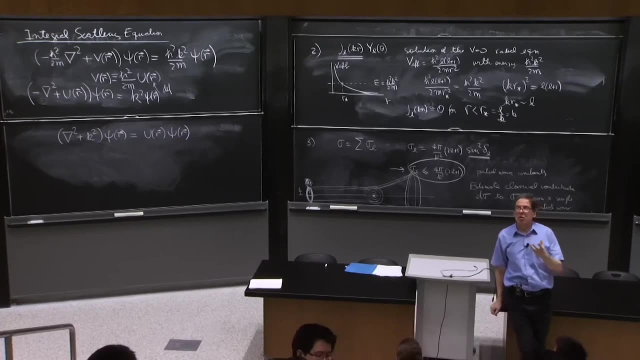 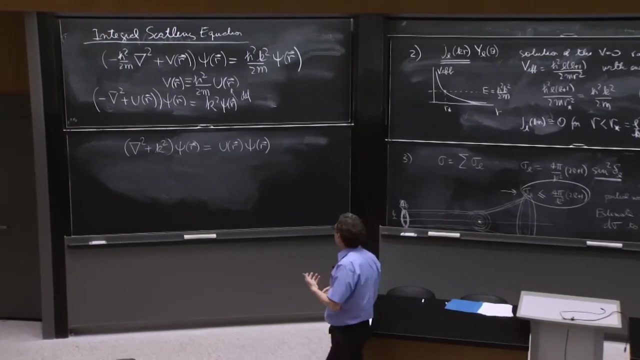 except put the equation in a way that stimulates our thinking. We kind of think of the right-hand side as a source and the left-hand side as a source- OK, And the left-hand side as kind of the equation you want to solve. 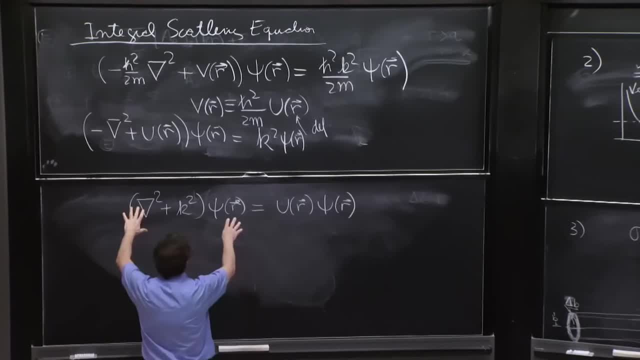 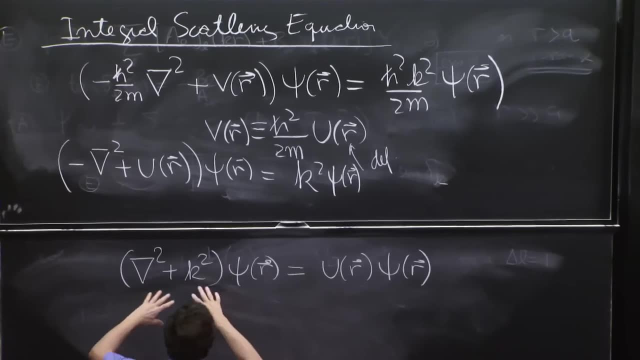 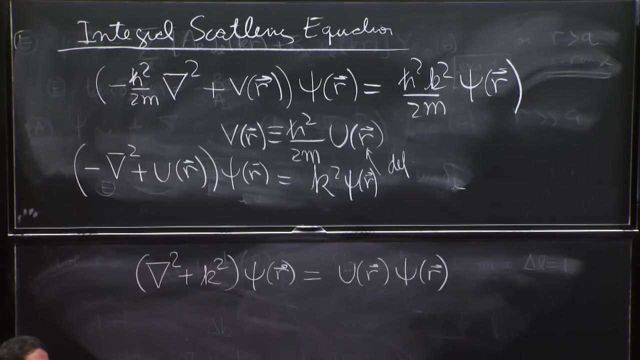 Sometimes you have an equation like that and you can get this 0 here. Well, that's when the potential is 0. But sometimes there's a bit of potential, so the solution feeds back into this. Whenever you have an equation of this form, some nice operator. 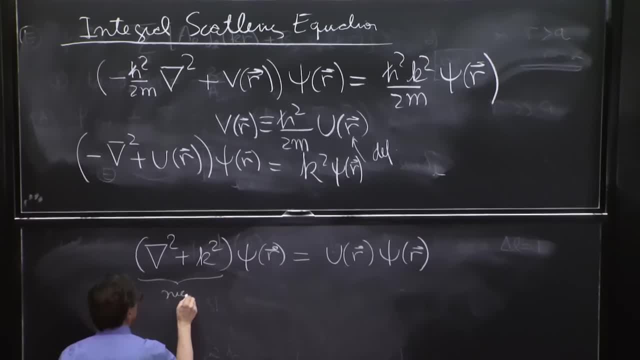 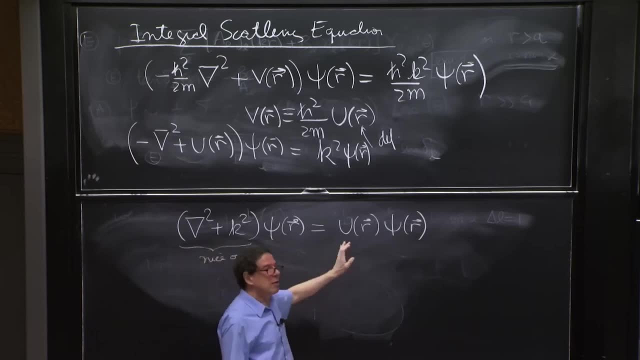 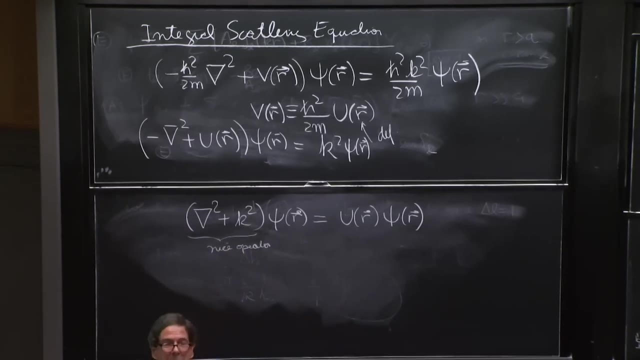 so this we call nice operator. It's acting on psi, giving you something that depends on psi. that maybe is not that nice or not that simple. We can try to solve this using a Green's function. That's what Green's functions are good for. 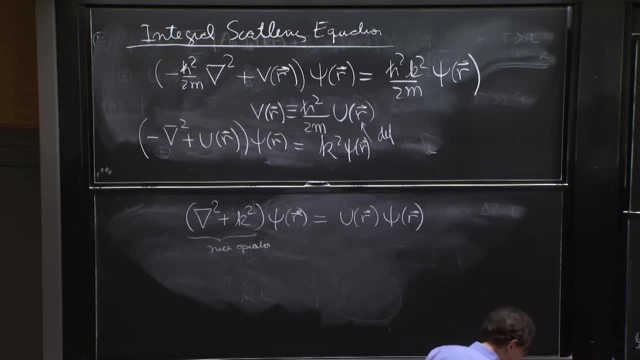 So let's try to use a Green's function. So what is a Green's function? It is basically Basically a way of understanding what this operator is. So nice operator must have a Green's function. So what is your Green's function here? 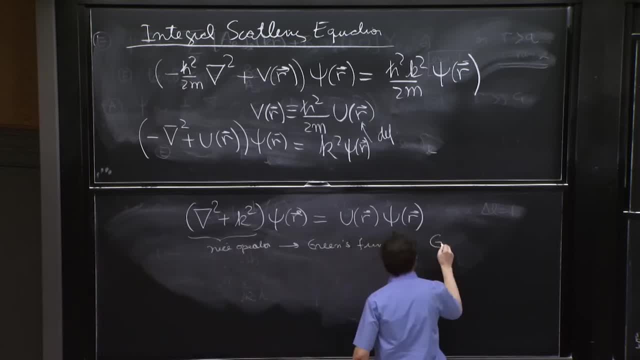 It's called G And we'll say it depends on r minus r prime. r prime is an rb, r prime is an arbitrary point so far. But here is what it does. It's basically a solution. You want this Green's function to be almost 0,. 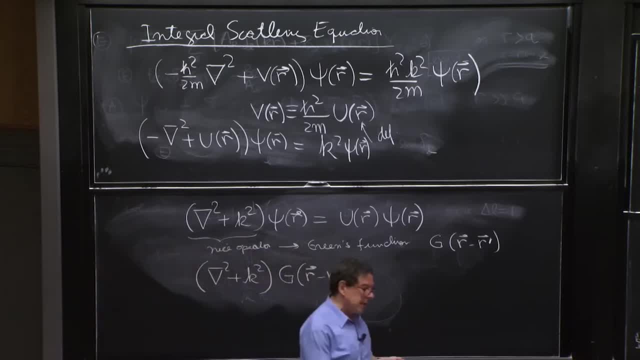 except they're not quite equal to 0. You want it to be equal to a delta. You want it to be equal to a delta function. So that's a definition of the Green's function. Is that thing which is the solution of a similar equation? 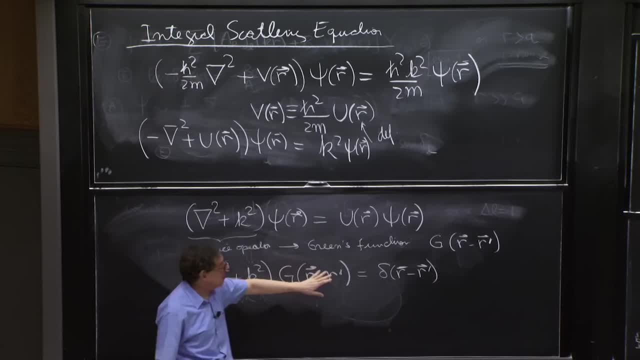 where you have the nice operator acting on the Green's function being just a delta function, It's almost saying that the Green's function is the thing that solves that equation with 0.. With 0 on the right hand side, Except that it's not really 0. 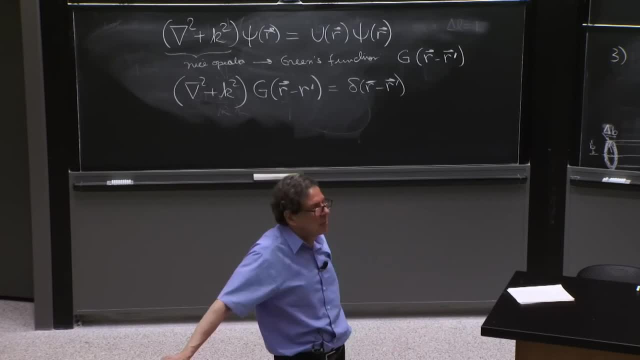 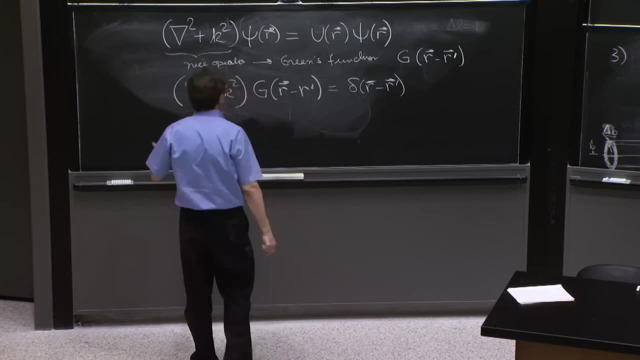 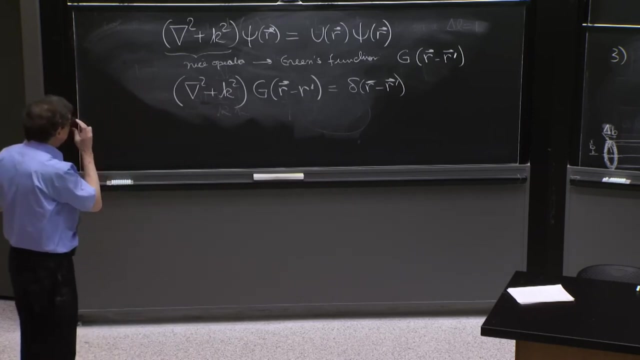 It's a source in the right hand side, It's a delta function at this point. So you would say maybe OK, I don't know Why would I care about this equation. You care for two reasons. The first reason is that this equation 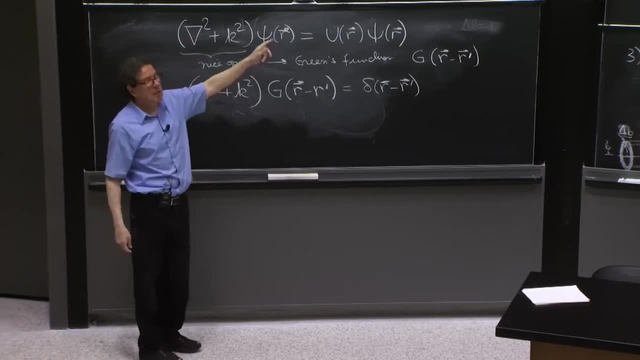 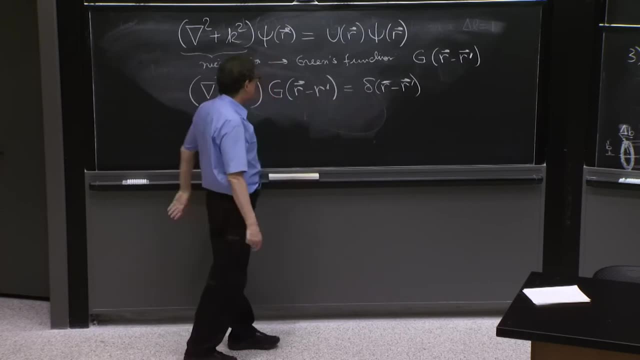 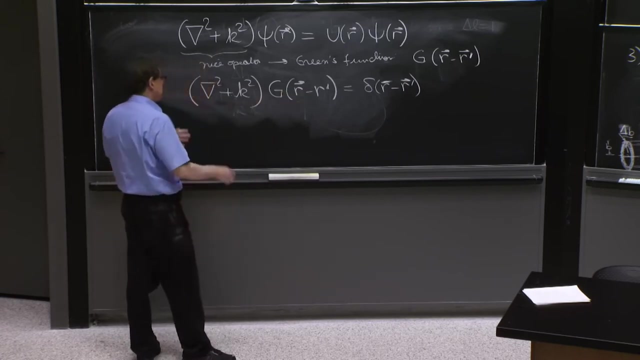 is easier to solve than this. one Doesn't involve the potential, which is complex. It's complicated, It just involves a delta function. So we can have this g and solve it once, because it doesn't involve the potential. And then the great thing about this equation: 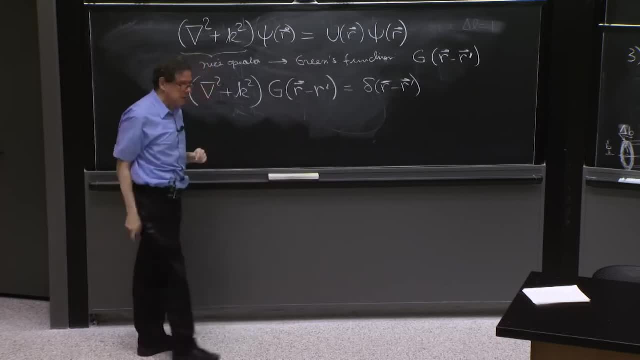 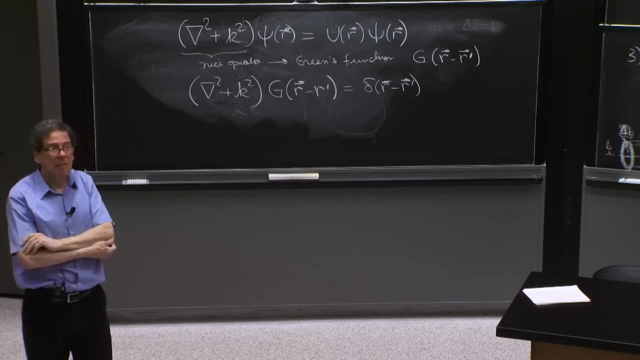 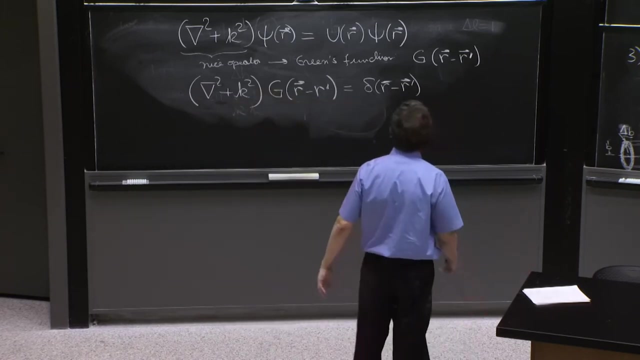 is that it allows you to write a solution for the top equation without having to do any work anymore. Once you have the Green's function, you're done. So let's assume you have the Green's function, How would you write the solution for this equation? 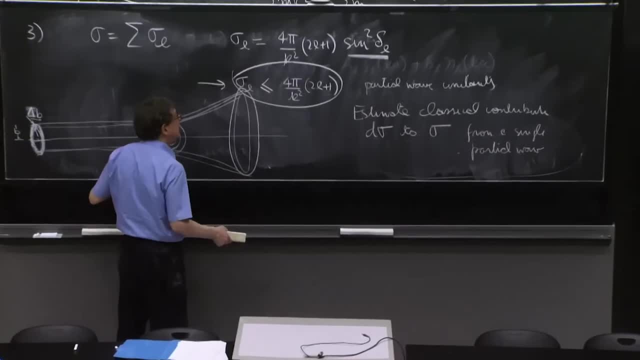 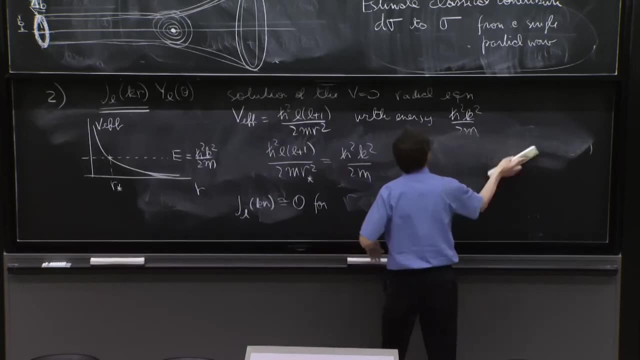 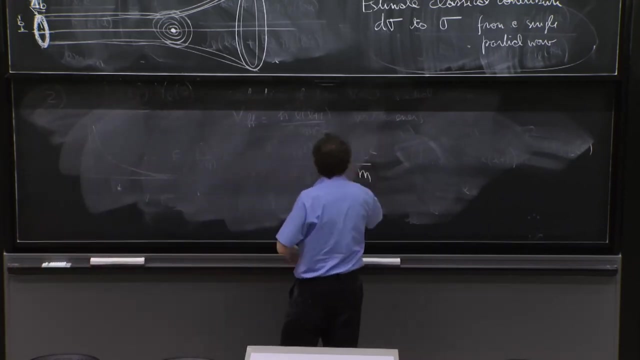 So the idea is superposition basically, And we'll do it using that. So our aim, We used to use superposition, Right, So let's assume we're on theıs superposition. So the idea is superposition basically, And we'll do it using that. 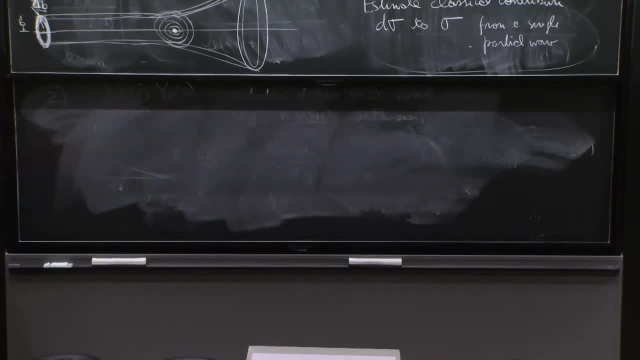 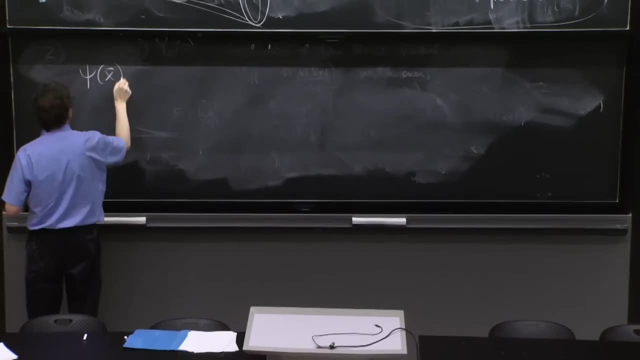 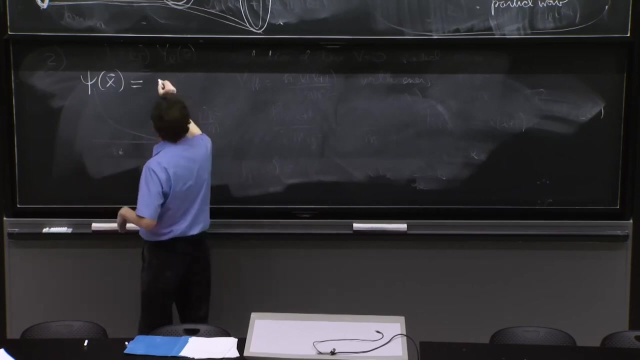 use this Green's function, if we had it, to write the solution for this equation. So here is the claim You write: psi of x is going to be given by a beginning one psi 0 of x. That is going to be a funny one. 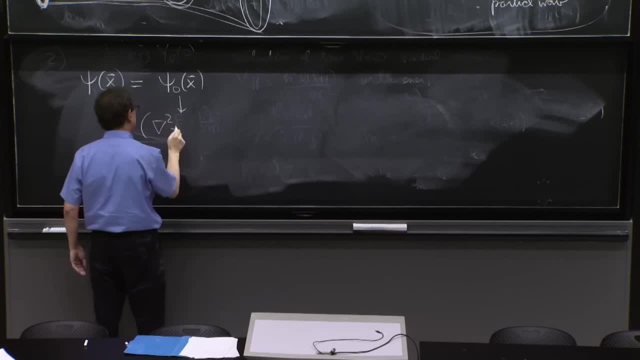 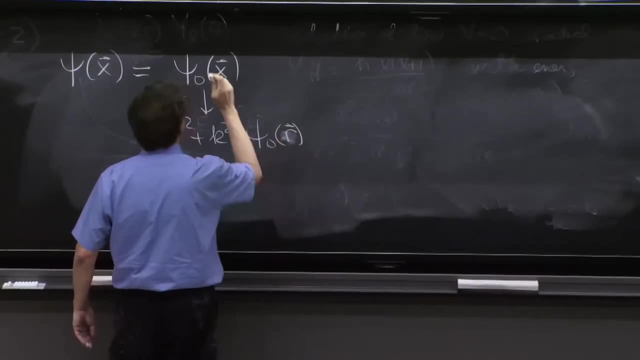 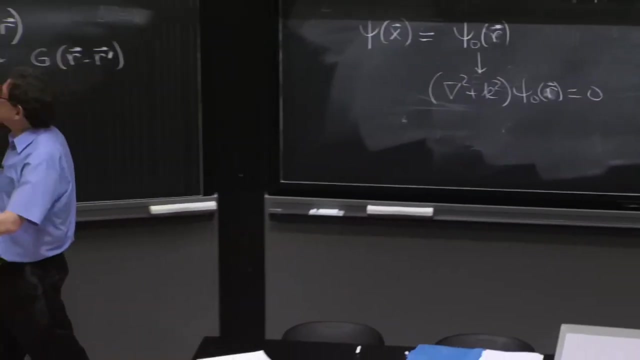 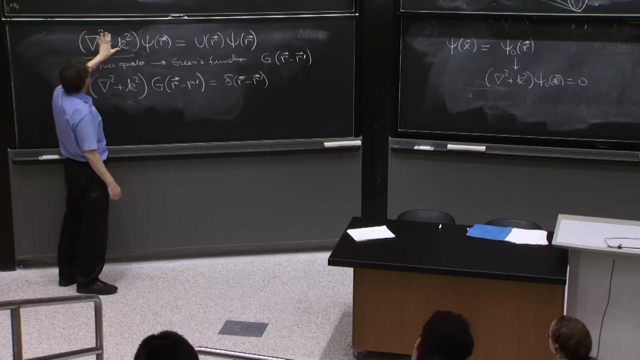 This one solves Laplacian plus k squared on psi, 0 of x or r is equal to 0. So whenever you have an equation of this form, you can add a solution. Anything that is killed by this can be added to whatever solution you have. 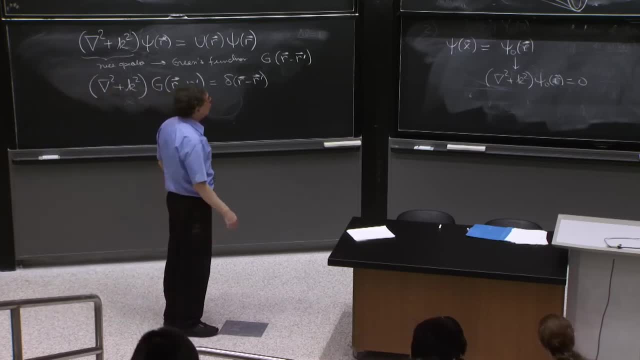 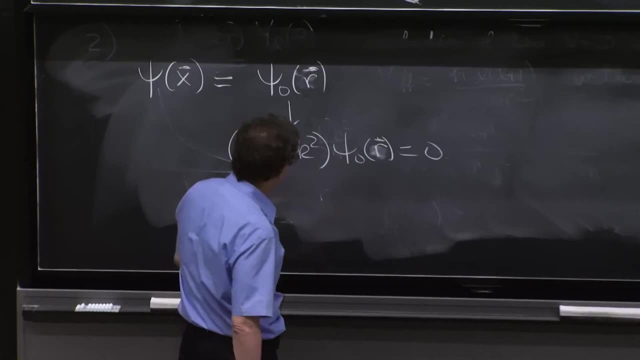 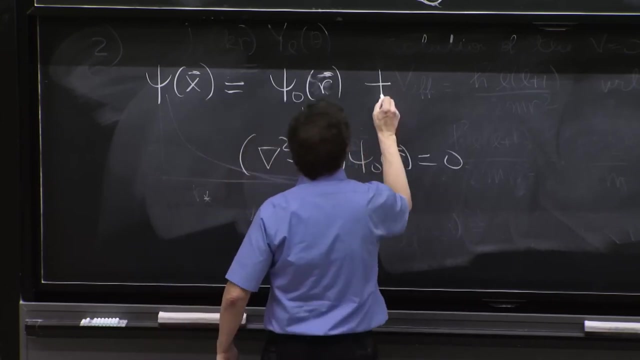 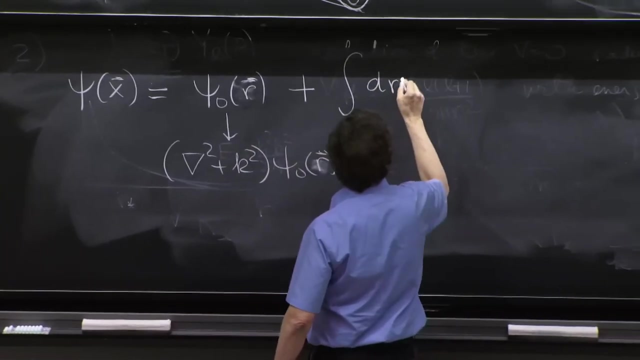 So. So let's assume that we have a solution of this form, psi 0, of this form. Now here I'll add one more thing. The important part is going to be an integral over r prime. Here is the superposition. 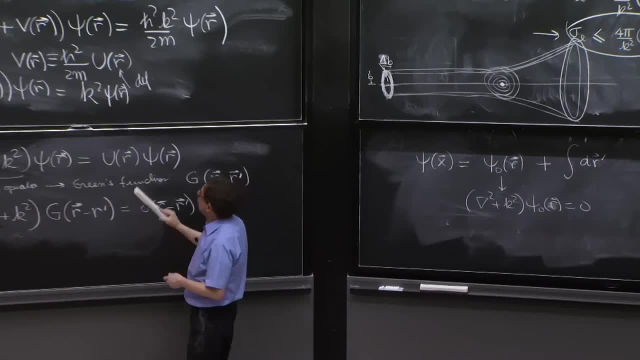 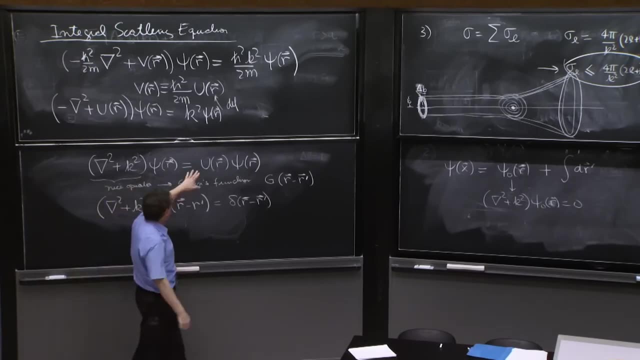 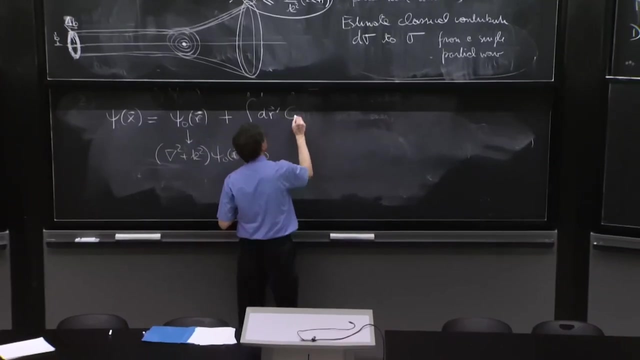 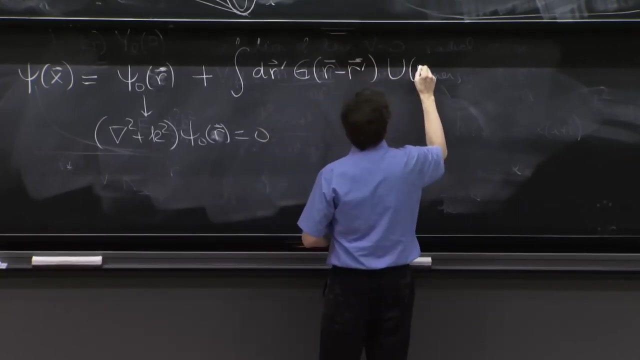 I'm going to think of this potential u of r. It's kind of existing at every point, r prime. So I'm going to write the solution as a superposition that involves the Green's function. So this will be g of r minus r prime times: u of r- prime times. 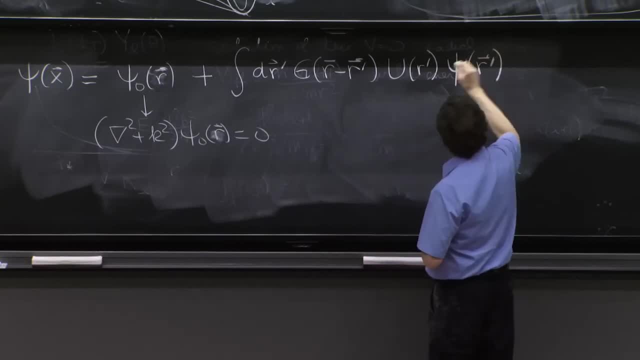 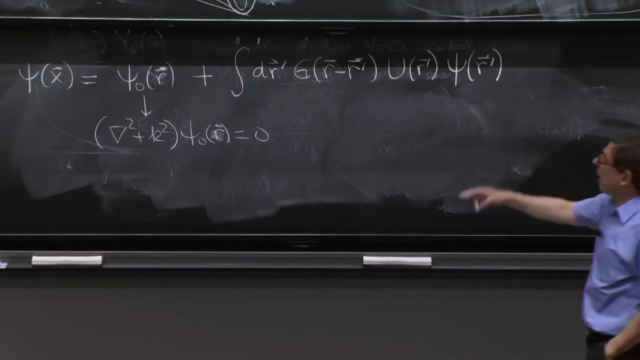 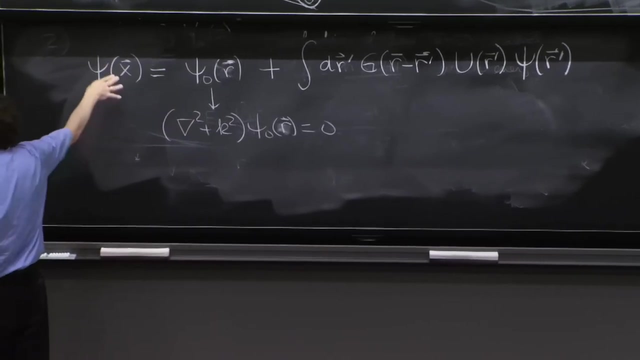 psi of r prime. I claim that this is equivalent to this equation that we have, that this psi provides more than equivalent. I think the precise way to say this provides a solution of this equation the way I've written, So let's try it. 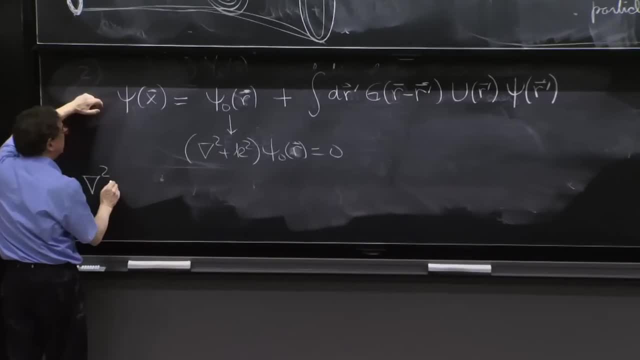 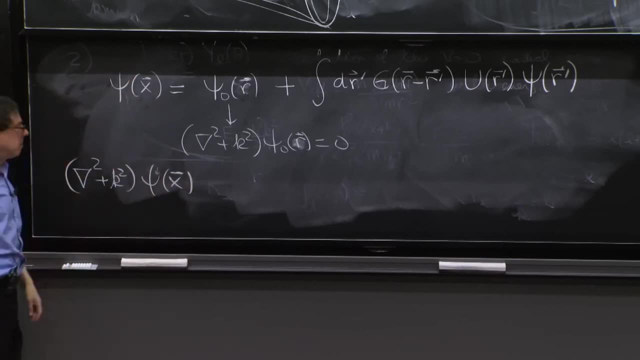 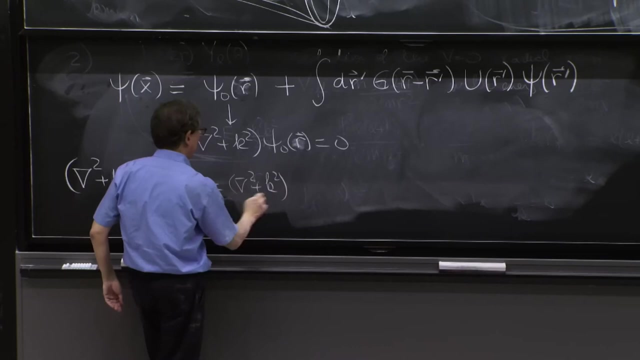 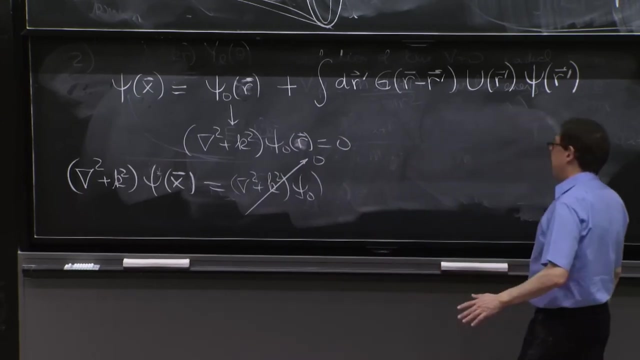 Suppose I calculate Laplacian plus k squared on psi 0.. So psi of x here, OK, The first term, it's already 0.. So Laplacian plus k squared on psi 0 is already 0.. And then I come here and I say: OK, I'm a Laplacian. 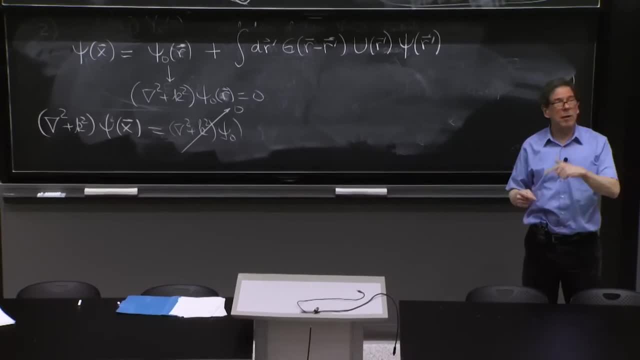 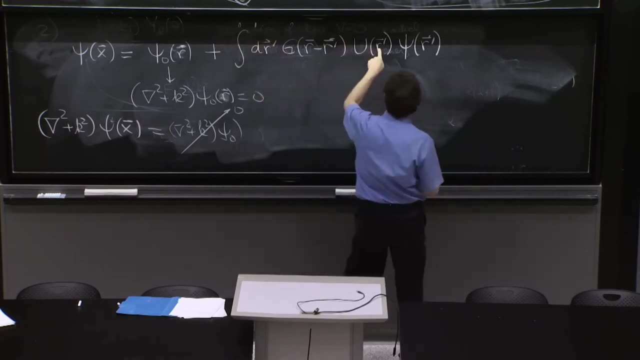 I care about r because I'm a Laplacian. I don't care about r prime. So I come in here And I ignore r prime, ignore r prime. I cannot ignore this thing. So we have plus integral dr prime Laplacian, plus k squared. 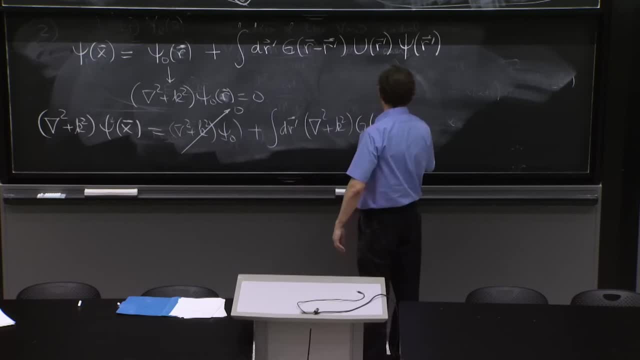 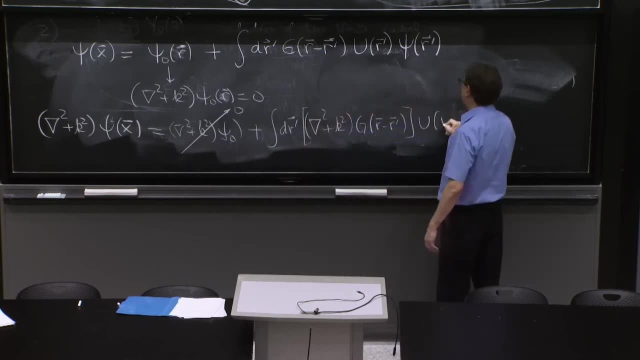 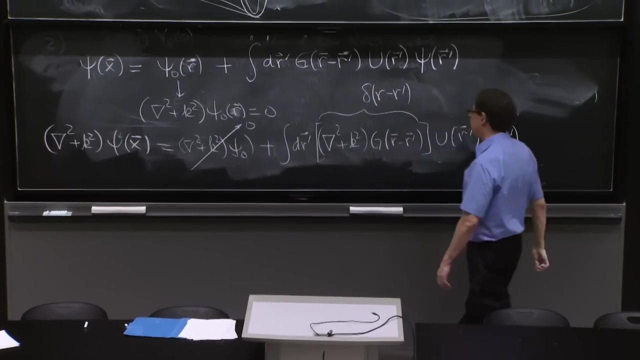 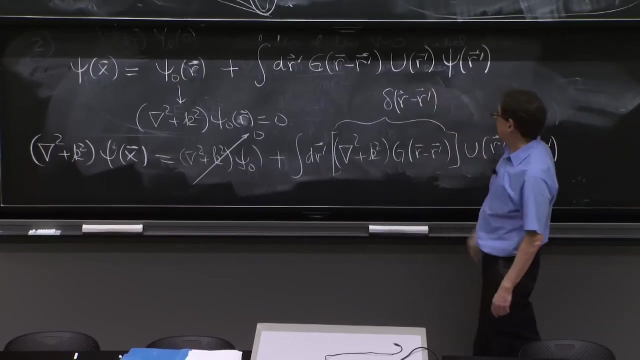 acting on g of r minus r prime, times u of r prime, Psi of r prime. And now, because the Green's function was designed to give you a delta of r minus r prime, this is an integral that can be done, the integral over r. 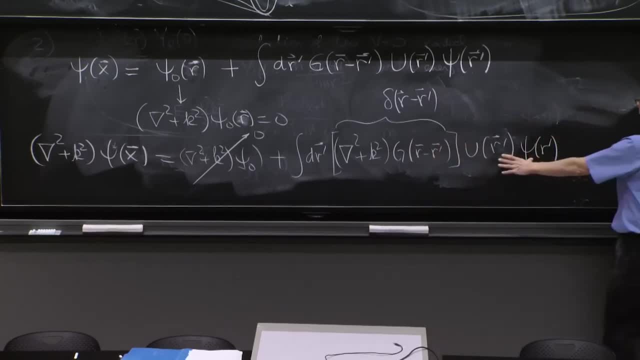 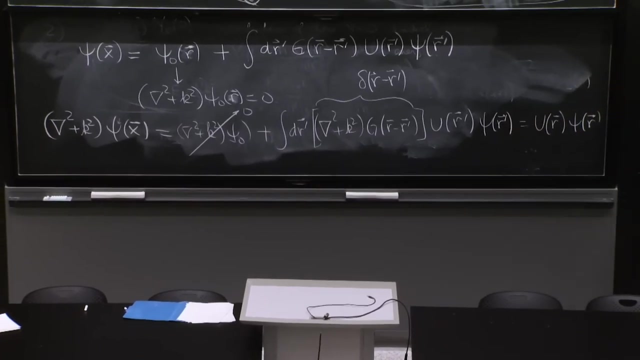 prime and just sets the rest, The rest of the integrand, at the point r, Because you integrate over r prime and this delta function fires when r prime is equal to r. So this gives me u of r, psi of r, And that is the equation I wanted to solve, the equation. 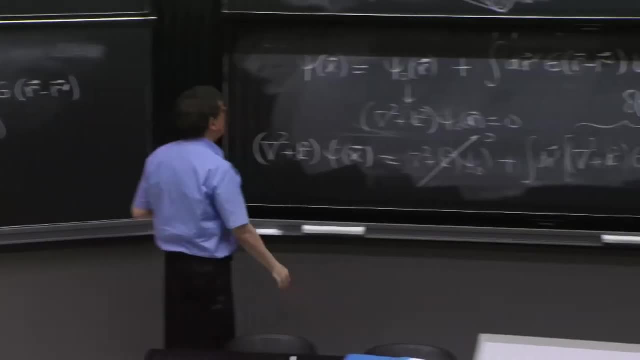 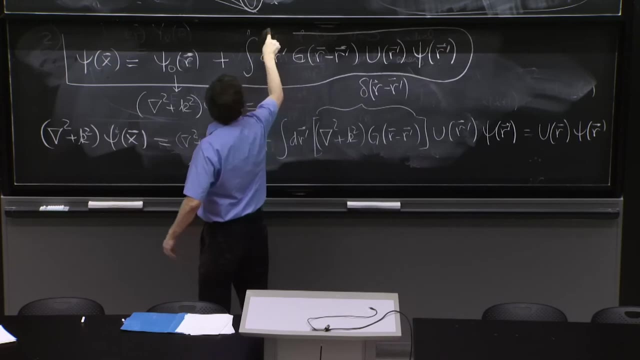 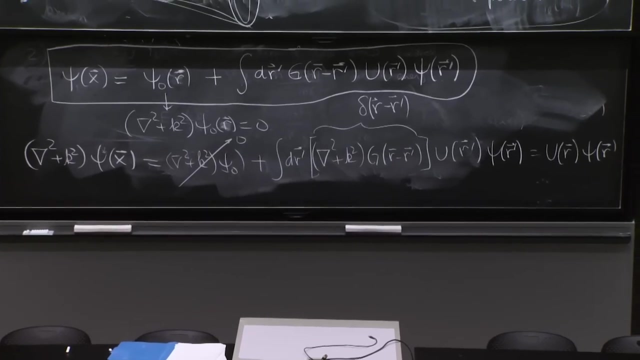 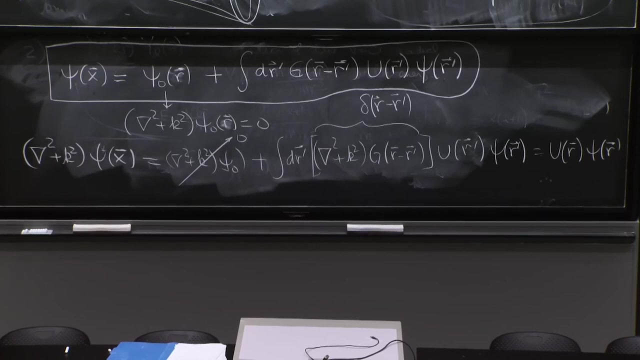 that we have here. So we have turned the problem. This cannot be called a solution because we have not solved it. We have turned the problem into a different kind of problem. We- it might even seem that we've made the problem worse by turning this. 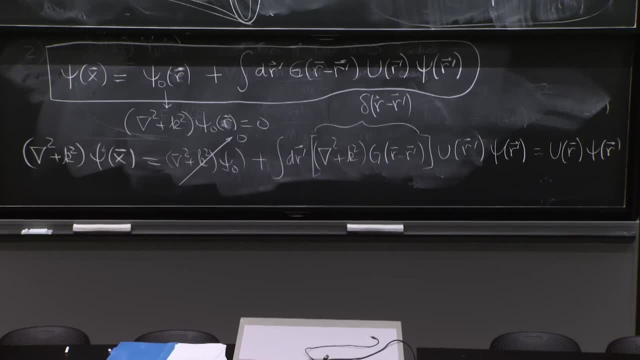 into an integral equation. There's no derivatives here, But the function that you're looking for appears outside and inside the integral. So these things are called integral equations, And the power of an integral equation is the insight it can give you, once you have an idea of what the Green's function is. 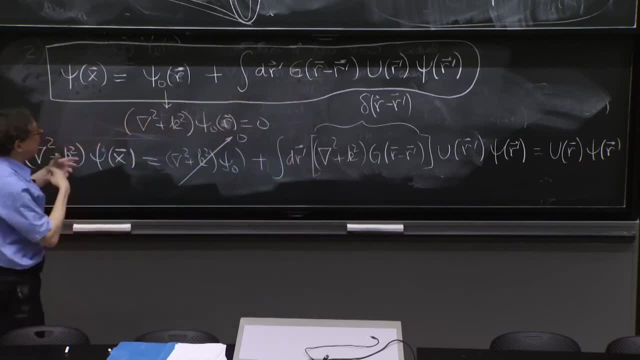 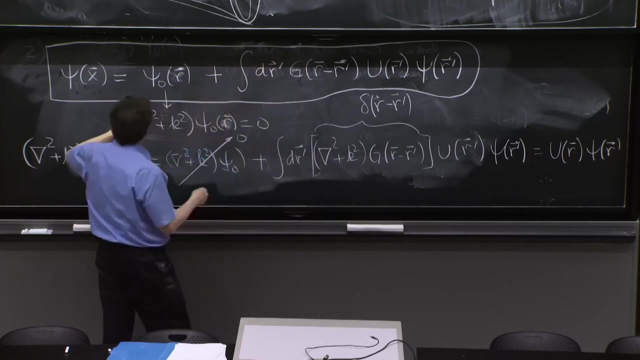 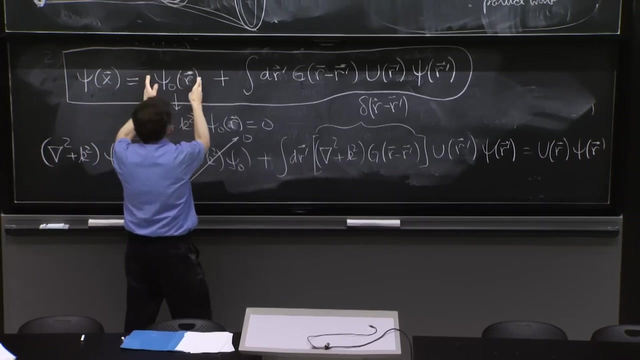 and also it's a good place to do recursive approximations, in that you can essentially begin and say: OK, I know the wave function is this plus that, but maybe, if in some sense I can think of this thing as the leading solution, I could substitute the leading solution. 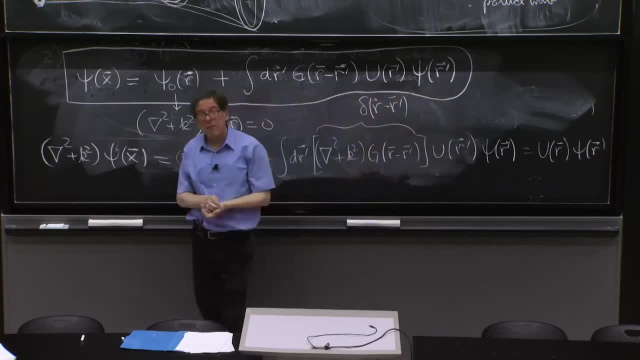 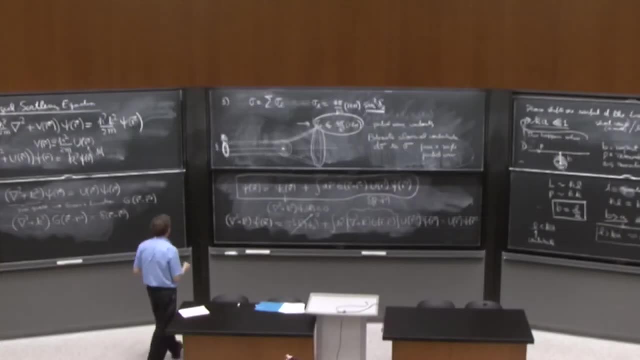 in here and try to make an approximation. That's going to give you a nice approximation. The Bohr approximation, The Bohr approximation. We'll see that soon. That should be all psi r's. I think I'm using r, So I please, so r's and r's everywhere. 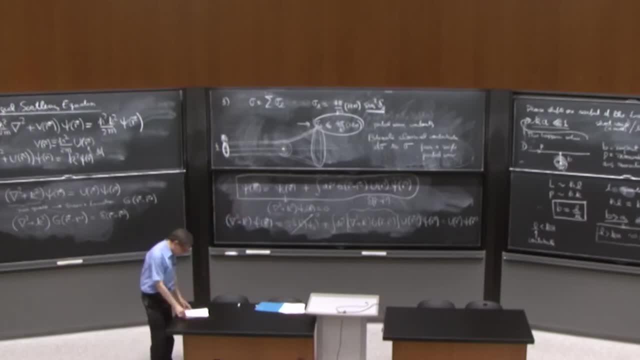 Yeah, no difference at this moment. OK, so the next step is solving for the Green's function. OK, OK, OK, OK, I need the Green's function, otherwise we kind of make progress with this equation. So I'm going to do a simple solution of the Green's. 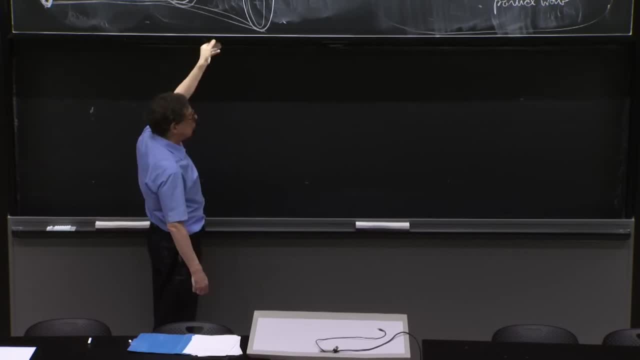 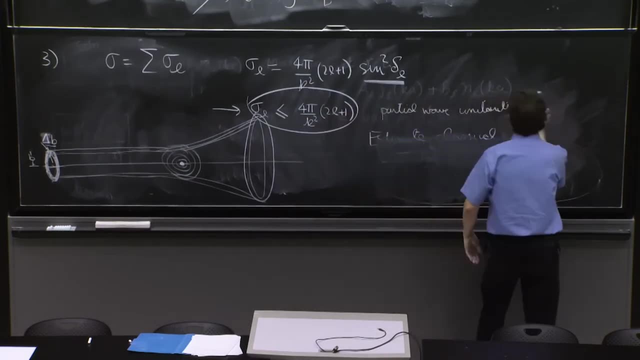 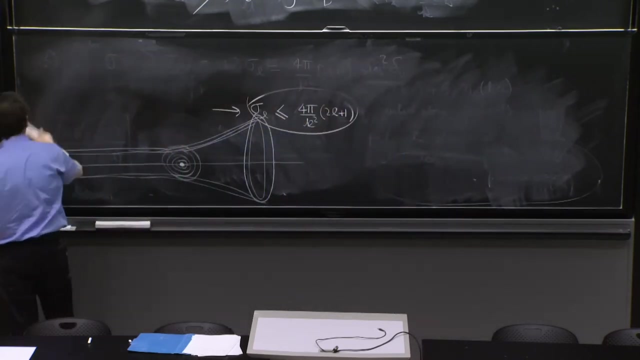 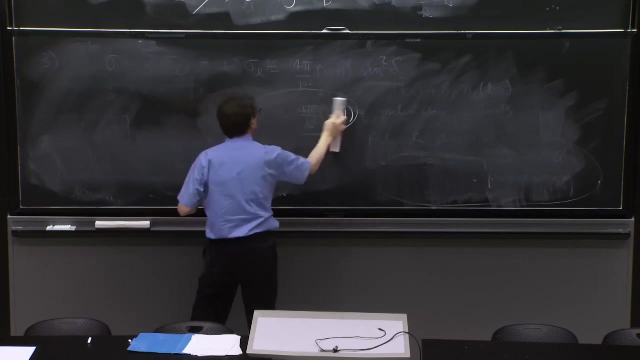 function, basically by doing a couple of checks and saying that is the answer we're interested in And there are several possible Green's functions and, depending on the problem you're solving, you choose the right Green's function And we'll choose the one that is suitable for us now. 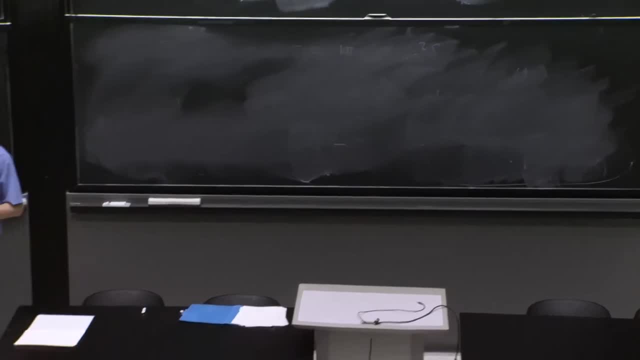 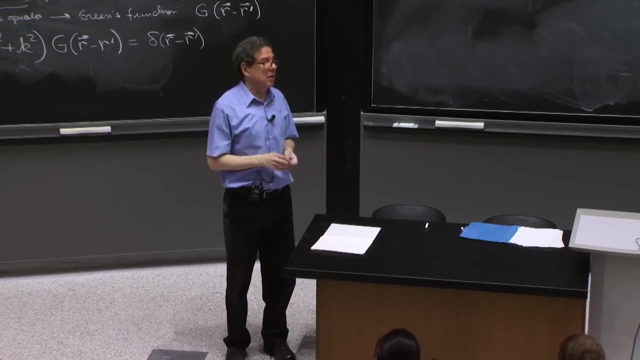 This is something that can be done. The general solutions can be obtained by contour integration, And there are all kinds of nice methods to do this, But in fact, in this case it's really simple. You don't need any of those complicated things. 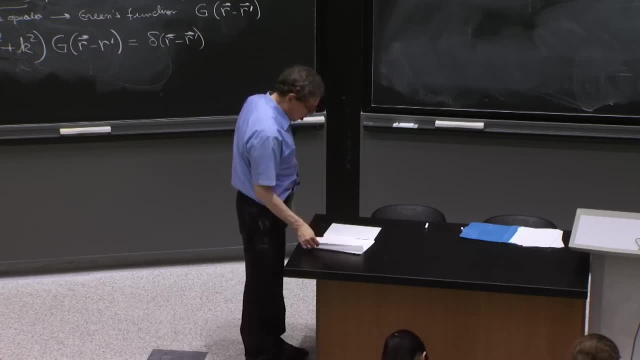 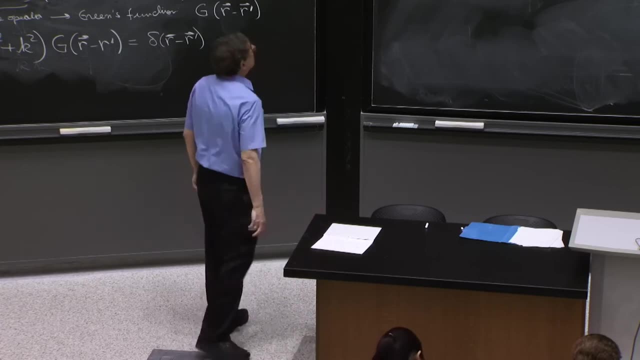 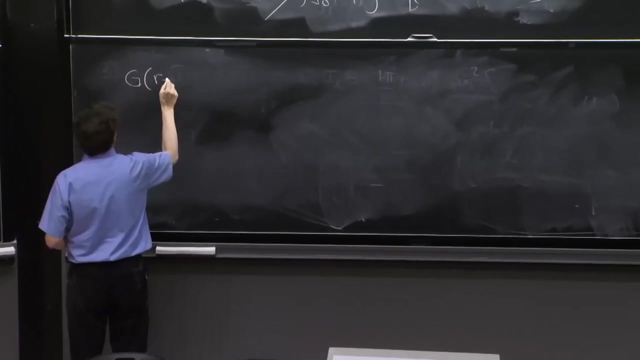 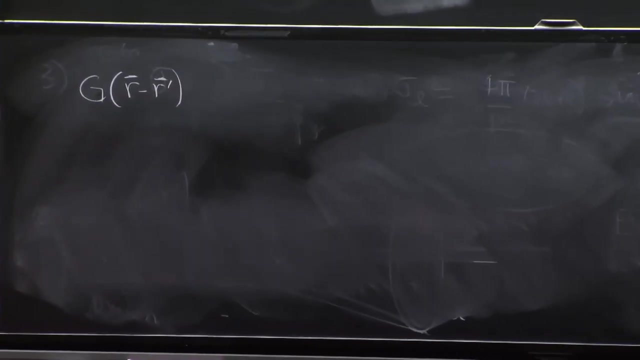 You can just pretty much write the solution, So that's what I'm going to do. So what do we need for the Green's function? So we have a Green's function that depends on r minus r prime, And so it depends on a vector. 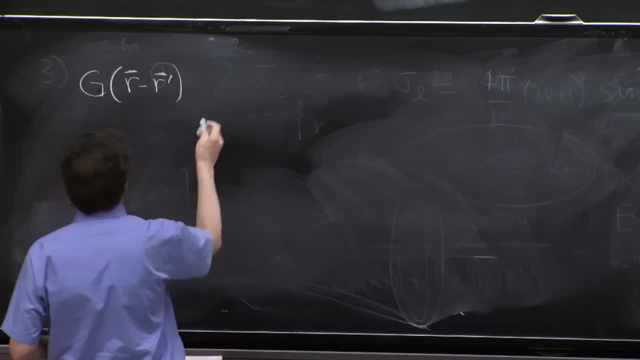 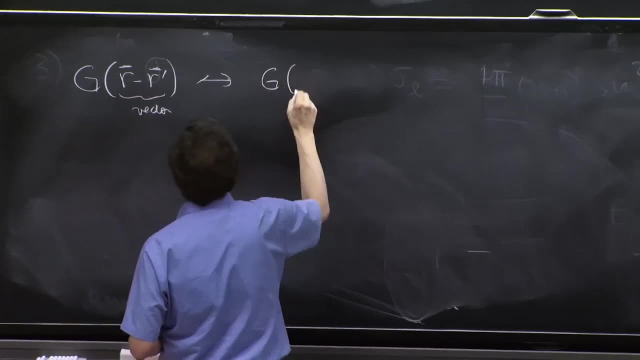 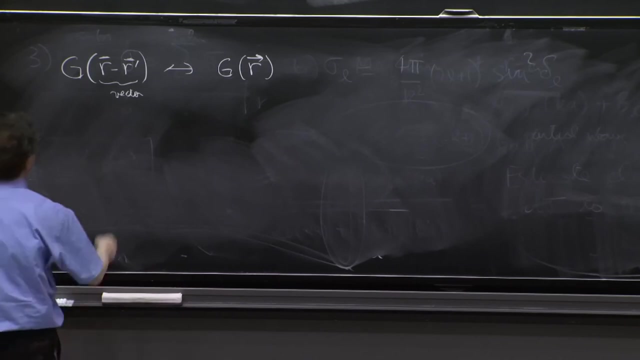 So let me simplify the matter by saying OK, since it depends on a vector, I'll just first calculate what is g of r, the Green's function of r, When the vector is r, or you could think it's when r prime is equal to 0. 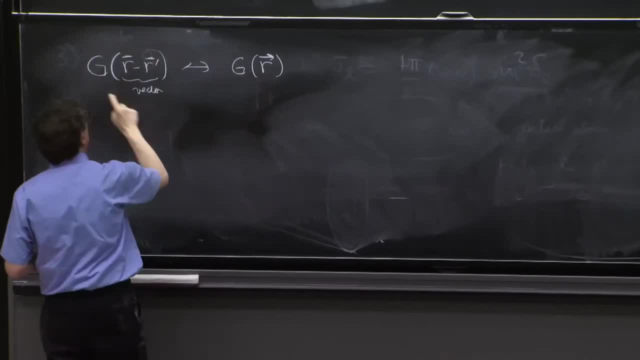 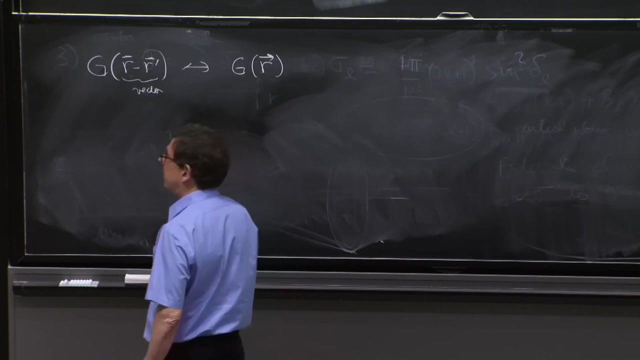 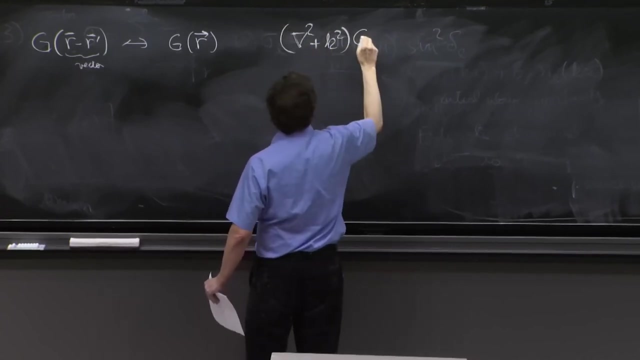 Whatever I find for g of r, this one is obtained by whatever I find here. put in instead r minus r prime. So g of r is enough for what we want to do. So it should have Laplacian plus k squared on g of r. 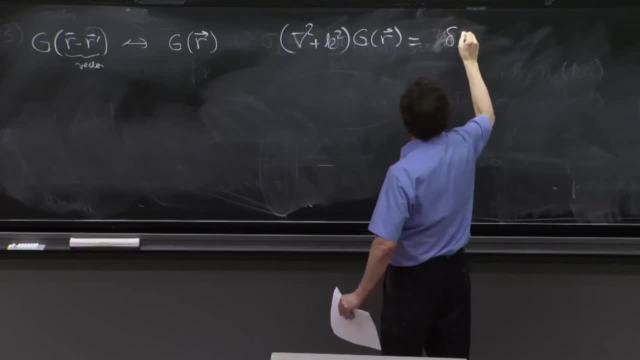 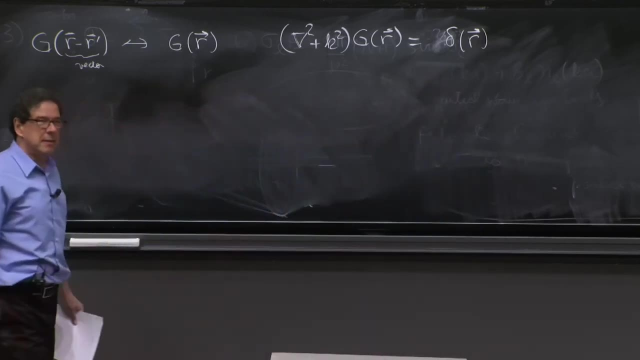 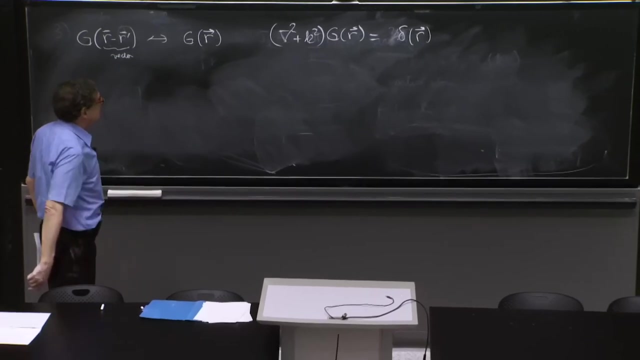 Should be 4,, not 4 pi. It's delta of r. OK, So we've looked at that. In fact, at the beginning of this course- not of this course of the discussion of scattering- We looked at this equation. 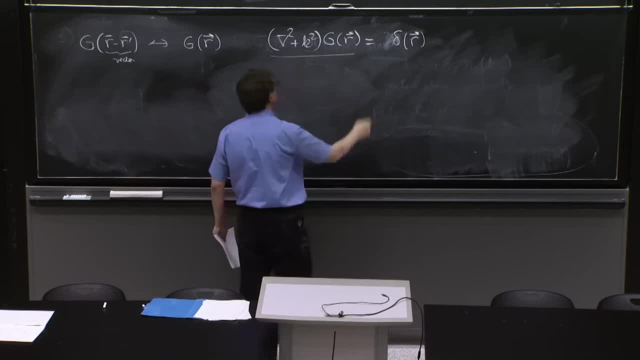 In fact we wanted to solve it when the right-hand side was 0, to find solutions of the Schrodinger equation, And we found that these g's could be of the form e to the ikr plus minus, ikr over r. Those were the spherical waves that solved this equation. 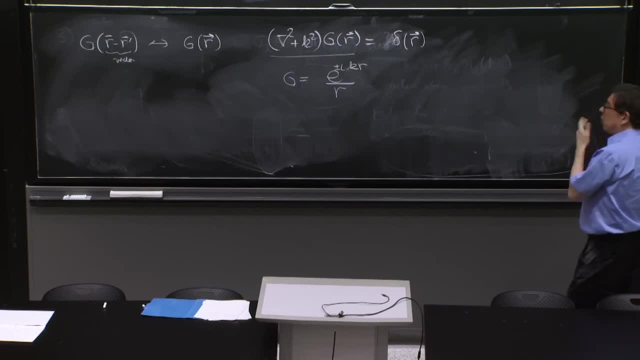 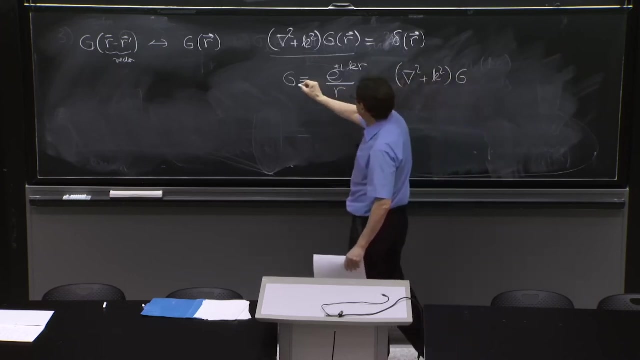 So we can do this with 0 potential. Those are our solutions. Now it's easy to see that Laplacian plus k, squared on this g that has a plus or minus, is equal to 0 for r different from 0.. The formulas for the Laplacian that you can use: 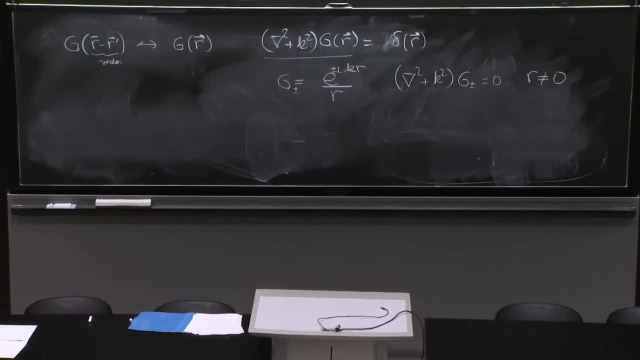 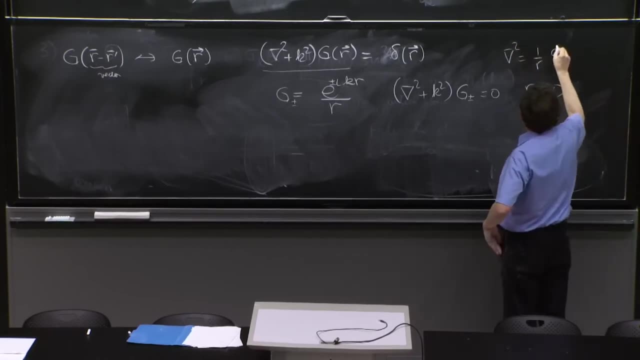 for r different from 0, you can check that is true And it's easy. You can use that formula, for example, that the Laplacian is 1 over r, d second. Well, it should be partial: d second, dr squared r. 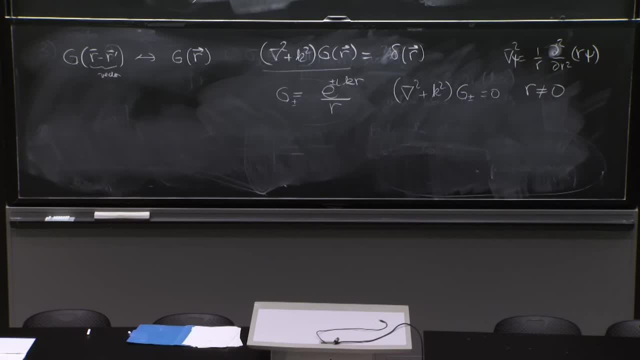 So psi, psi, Like that That formula in 1, 30 seconds you can see that that works for r different from 0. But then you can do this. And then there's also a formula that you know, that Laplacian of 1 over r from electromagnetism. 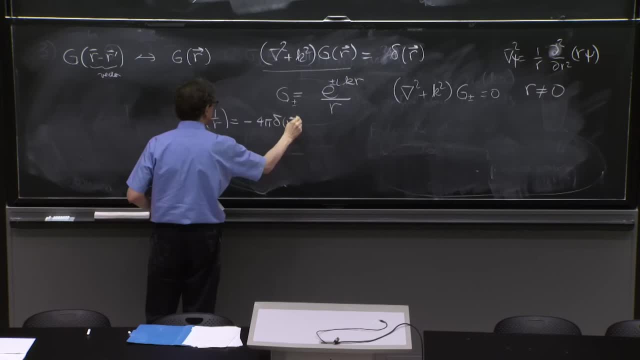 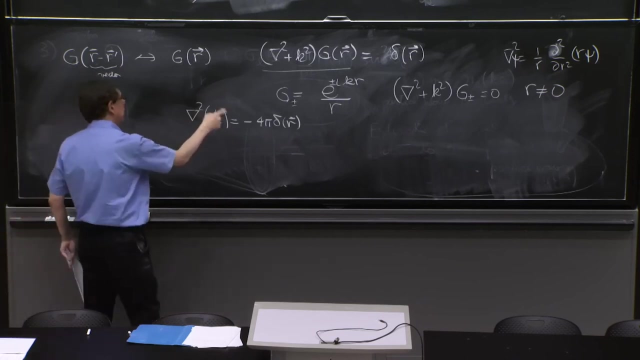 is minus 4 pi times the delta function of r. This comes from Poisson's equation in electromagnetism. So that's saying Laplacian of the potential is the charge density. This is the potential for a charge. The charge is at r equals 0.. 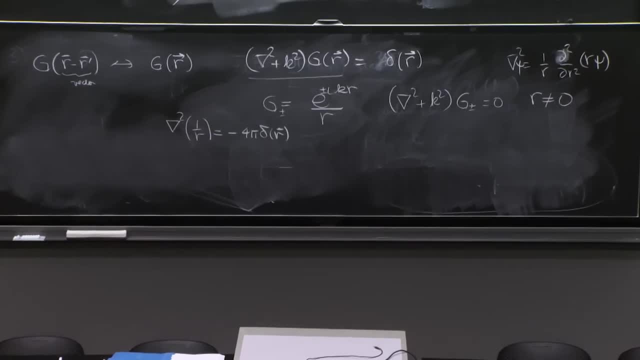 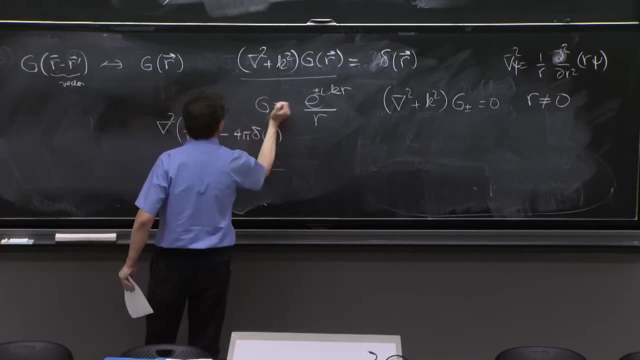 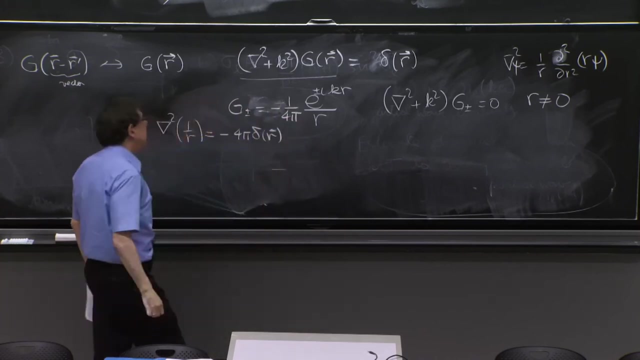 It's a singularity, It's something you study. So here, if I put a minus 1 over 4 pi for g plus minus a minus 1 over 4 pi, the Laplacian of this whole thing is 0.. 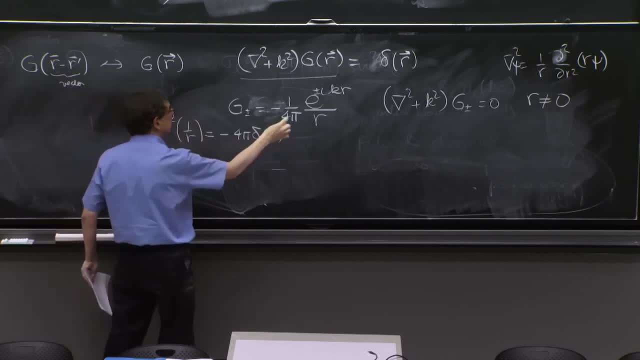 But when you approach 0, the Laplacian of this function, this function approaches just 1 over r, As r goes to 0, this goes to 1.. And the Laplacian of 1 over r gives you this minus 4 pi. 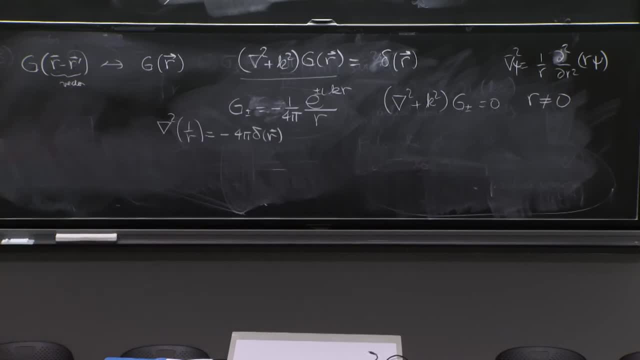 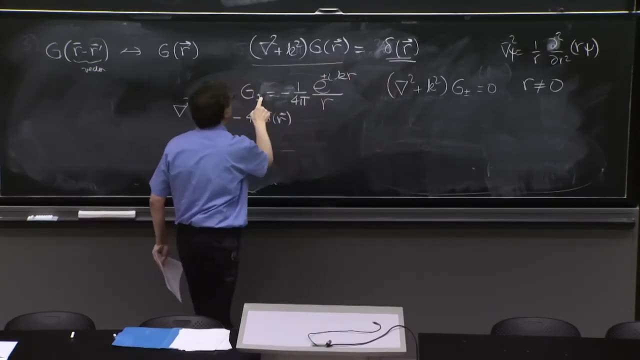 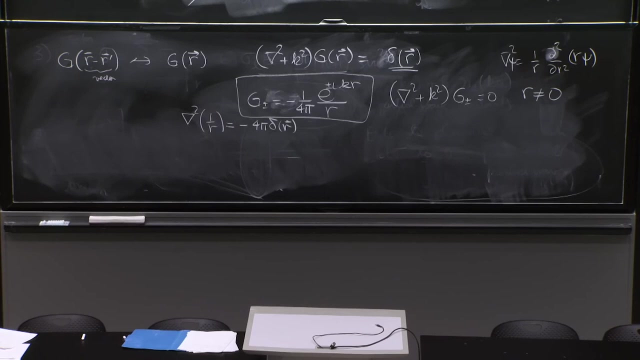 cancels with that And it will give you a delta function. So the delta function will arise correctly from this quantity. So I've argued, without solving this equation, that this this does give you a solution for the Green's function. It's Laplacian plus k. squared is 0 away from 0.. 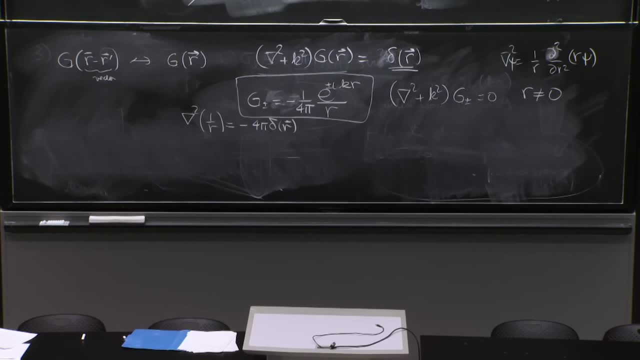 And as you approach 0, it has the right singularity to give a delta function. So this is your Green's function. As I said, many ways to derive it If you want. see Griffiths, see other ways in which it's done. 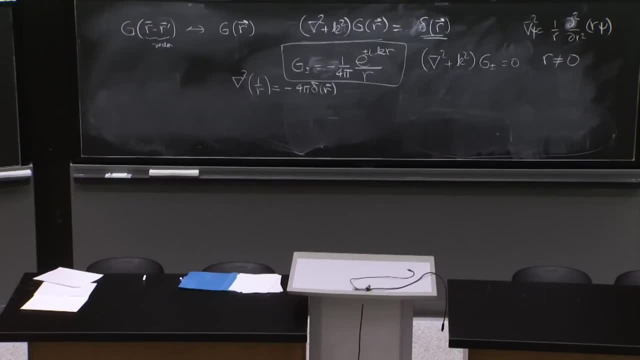 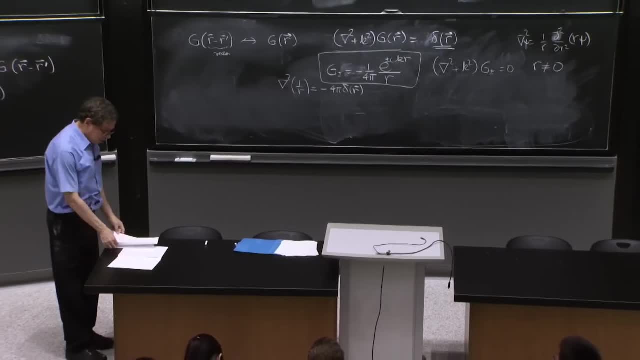 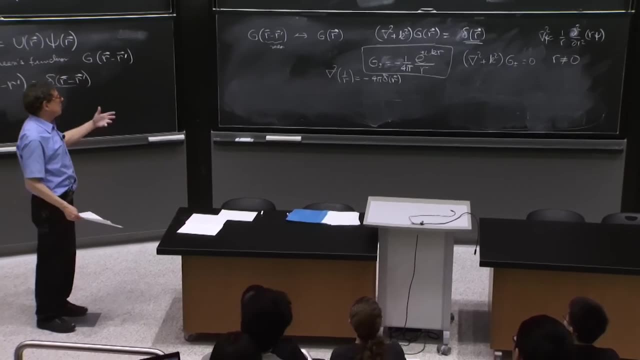 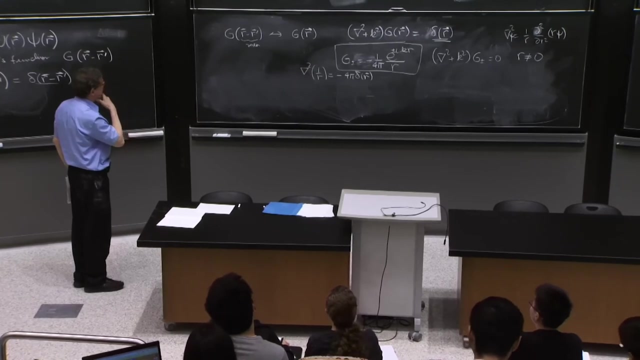 It's very simple. Then you can also check this by doing properly the vector calculus. You can take a Laplacian as divergence of the gradient and calculate every step, And it's fun to do it as well. You check that this works. 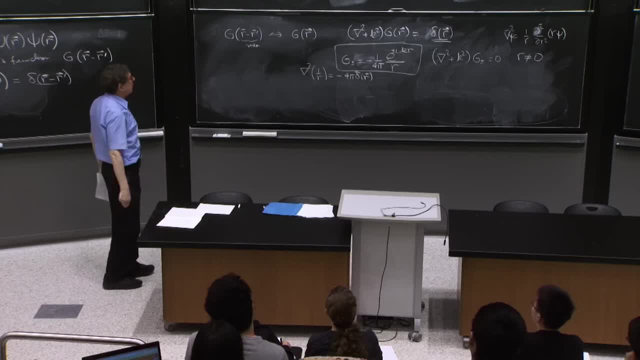 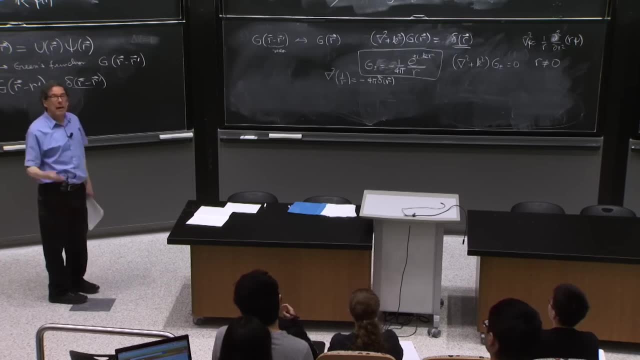 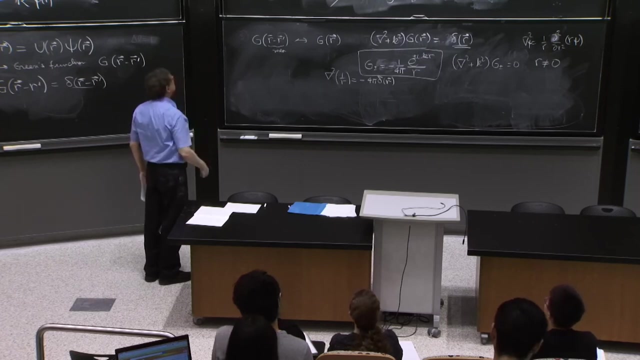 So this works And now we have to make choices, And our choices are going to be adjusted, adjusted to the problem we're trying to solve. We're trying to solve a scattering problem and psi 0 represents a solution, And from the way we thought of our waves, 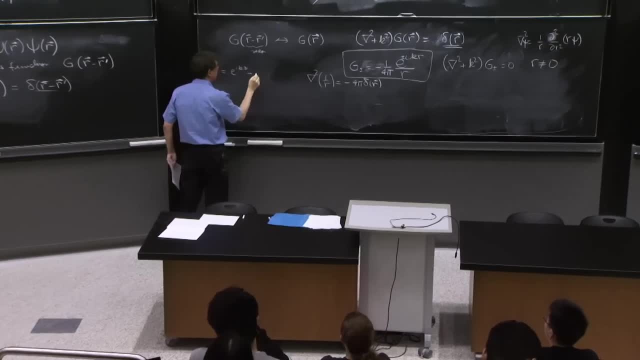 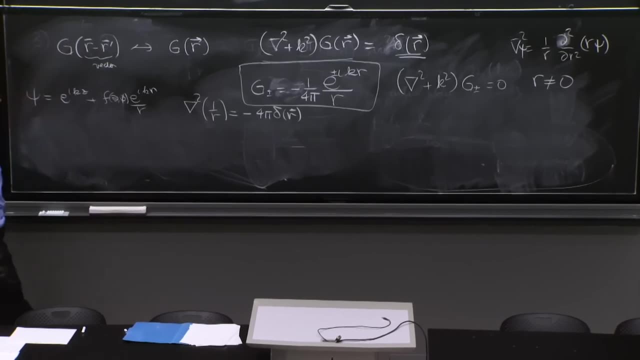 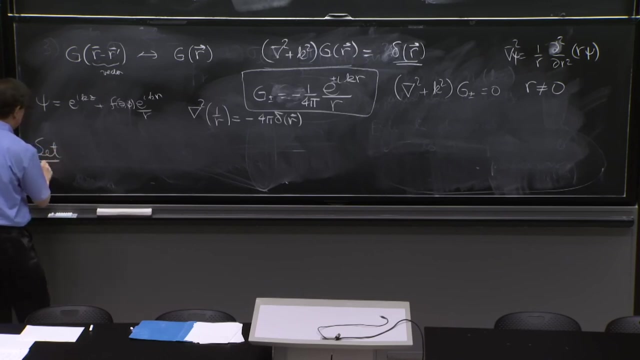 we had psi equal e to the ikz plus f of theta and phi e to the ikr over r. So it's reasonable to try to set- And we're going to find solutions- by setting psi 0 to be e to the ikz. 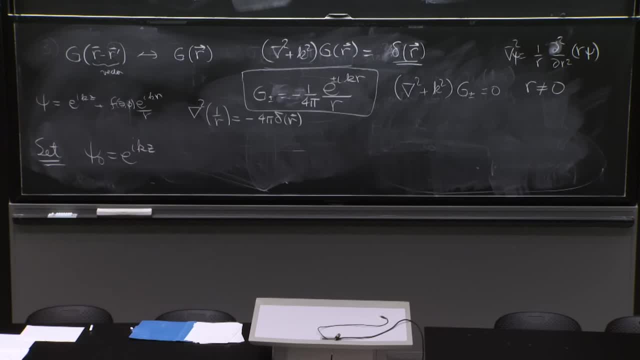 It does solve the equation: Laplacian squared plus k squared equals 0.. And then we're going to set the Green's function to be g plus with a plus here, because we want solutions. We want solutions of the type e to the ikr. 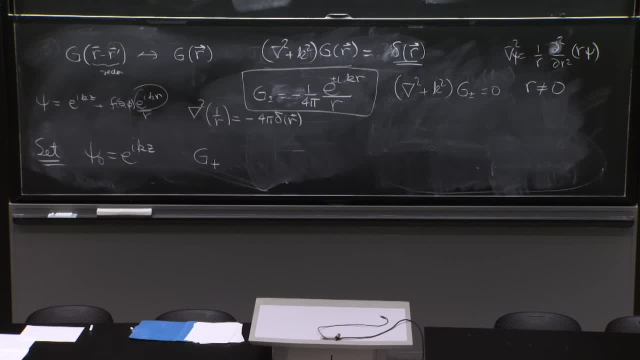 We've already decided those were the solutions we need, And a Green's function with a plus in there is going to generate that. So those are fine. You could have chosen another thing here, an arbitrary solution, And you could have chosen a g minus as well. 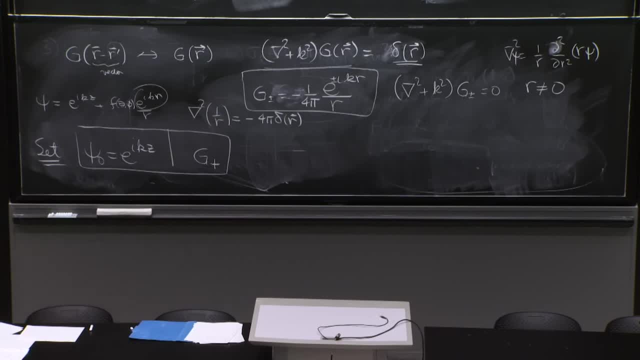 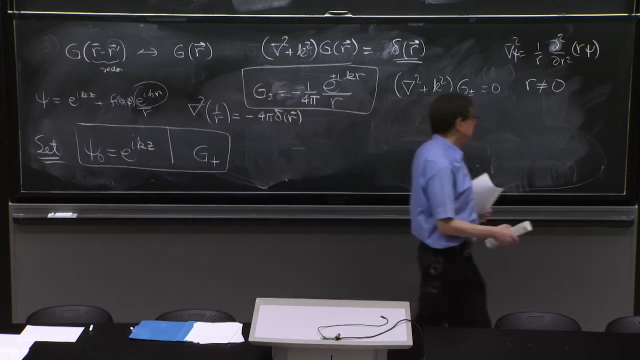 And you would get a solution of the Schrodinger equation, But it would not have much to do with the solution we're trying to get. So let's show that this gives us this kind of solution we want to get and gives us already a formula for the scattering amplitude. 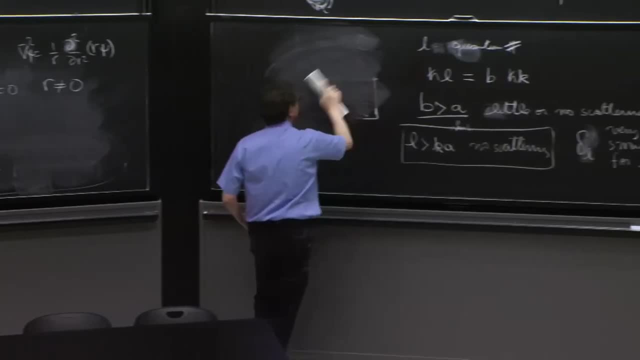 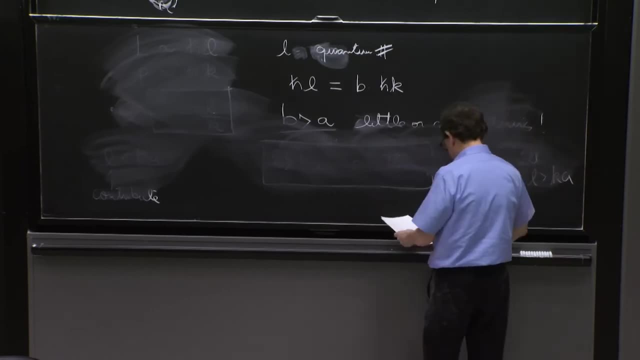 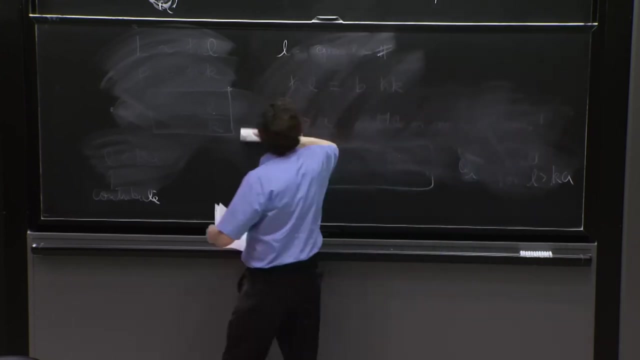 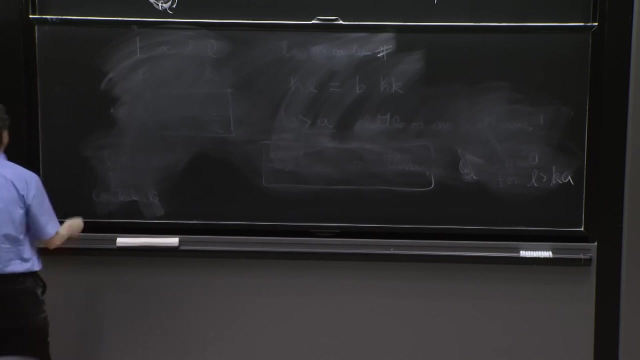 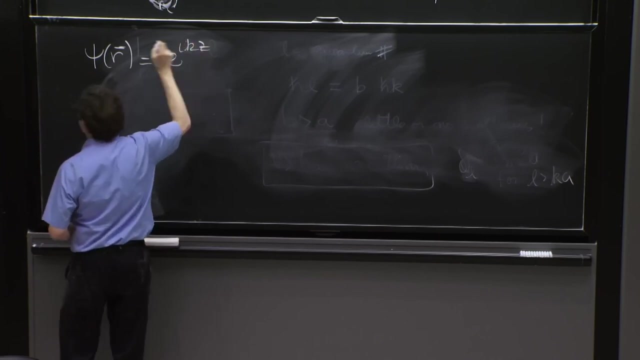 So let's do that. For that we just need to write what the Green's function is and approximate, So it will be a first step. OK, So what do we have? Psi of r is equal to e to the ikz. 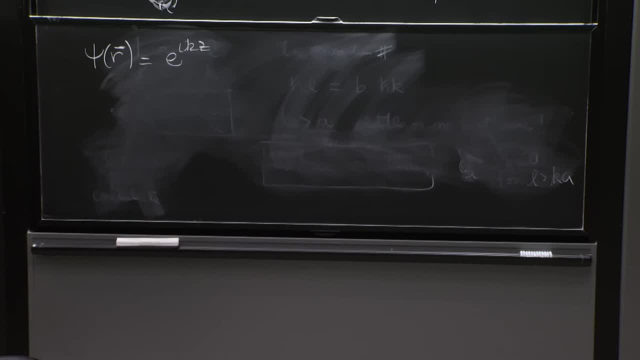 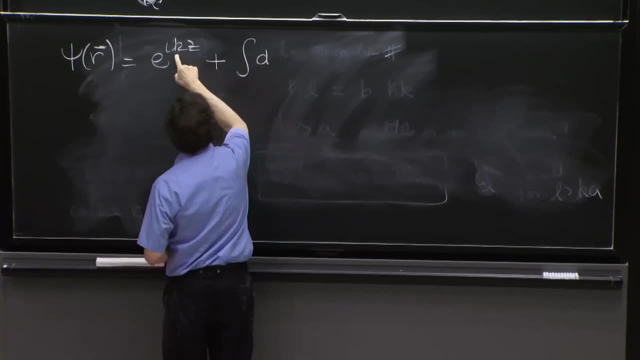 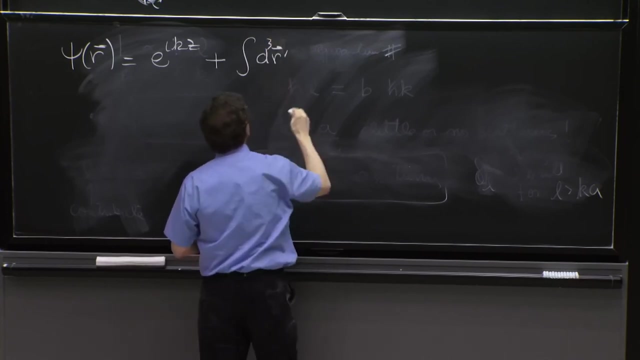 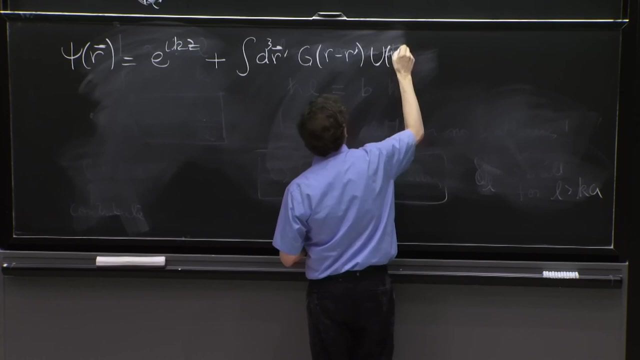 I'm writing up this top equation, But we now write it with the right boundary conditions, which correspond to a psi 0.. And a particular choice of the Green's function: d cubed r prime. g of r minus r prime. u of r prime. 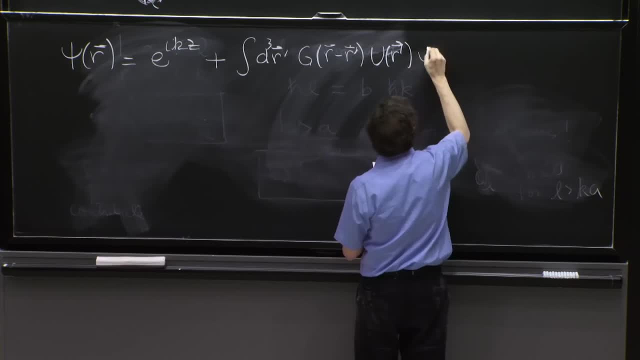 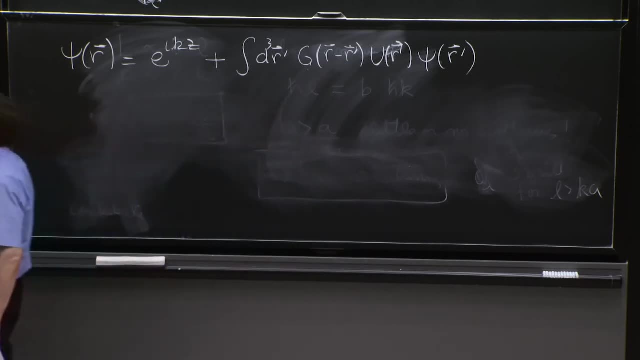 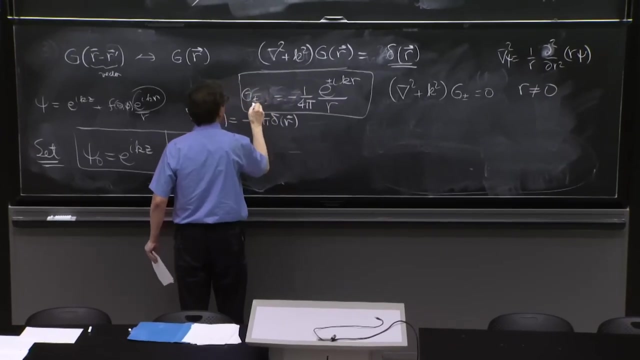 All those are vectors. And psi of r prime, All those are vectors, except g, which is pretty in that it is spherically symmetric. This g plus r prime, It's a vector. This g plus minus of r just depends on the magnitude of r. 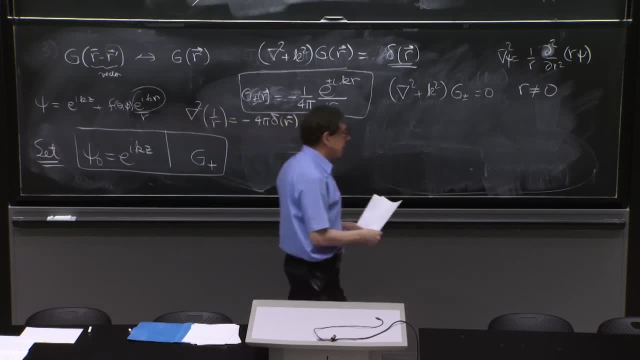 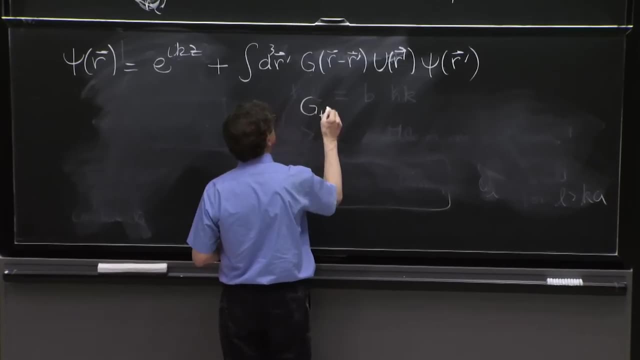 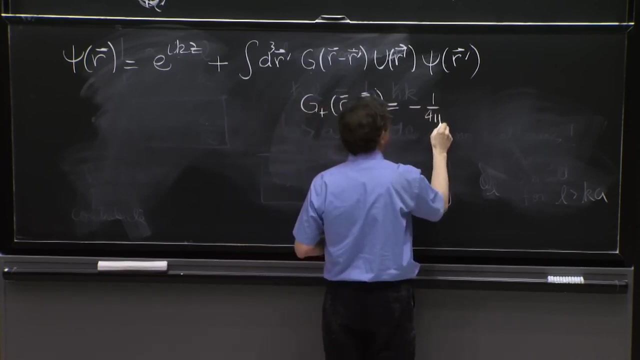 which is very nice. OK, So a couple of things that we can do here and most everybody would do. Let's g plus of r minus r prime is equal to minus 1 over 4 pi e to the ik Length of r minus r prime. 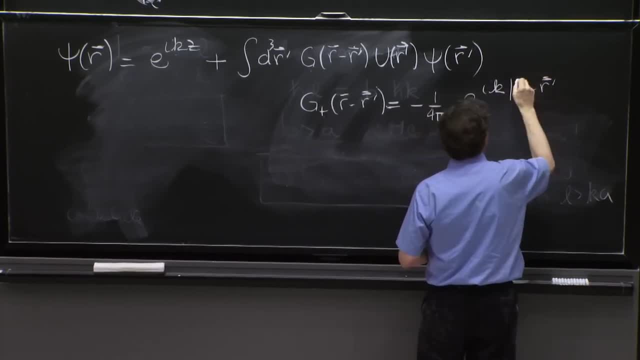 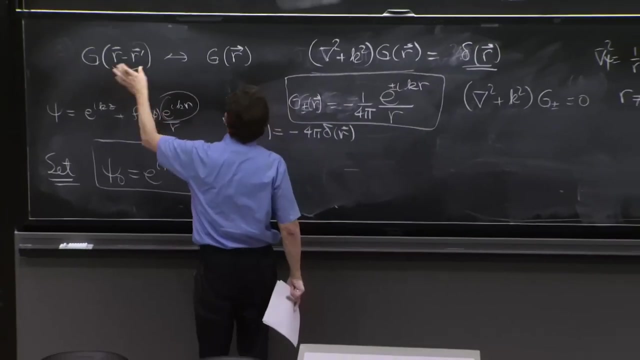 Let's write that down. Let's write that down. Length of r minus r prime. That's what this is supposed to be over. length of r minus r prime. Remember I said to you that whenever we had g of r, then to get the one we need, we'll. 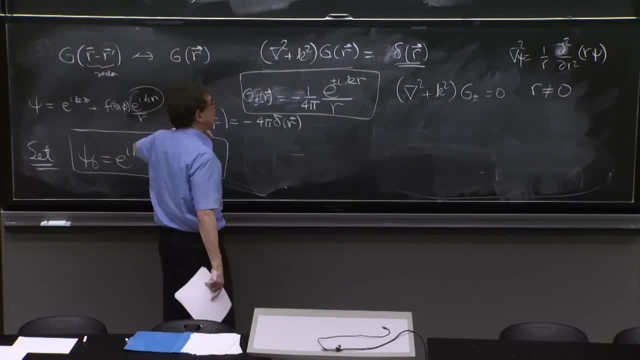 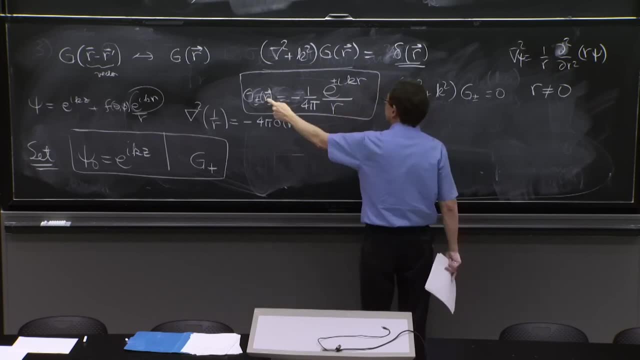 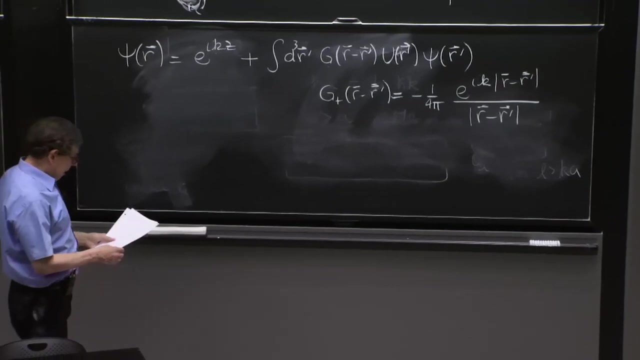 just have to replace the r by r minus r prime, And here this little r or r without the vector is the magnitude of this vector. So we've put the magnitude of those vectors. We've put the magnitude of those vectors there. 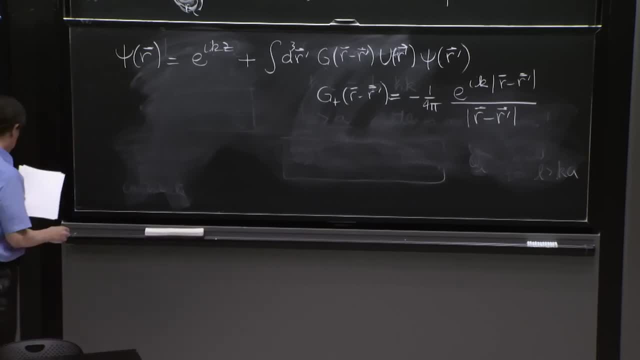 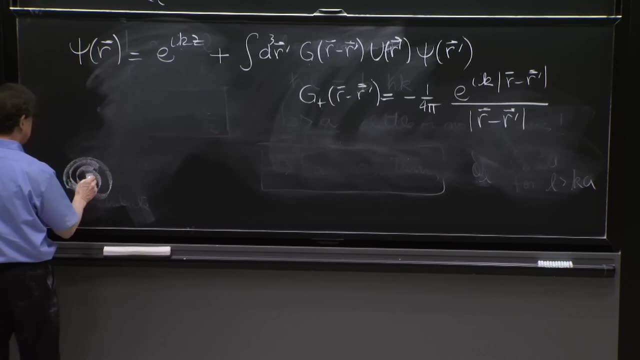 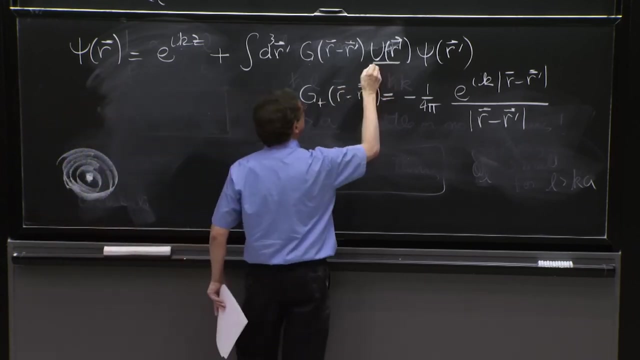 Now people look for approximations in here. So here is what we need to do. Imagine the origin. here is a potential and you have your system of coordinates. You are integrating over places where the potential exists. So the r prime that you're integrating. 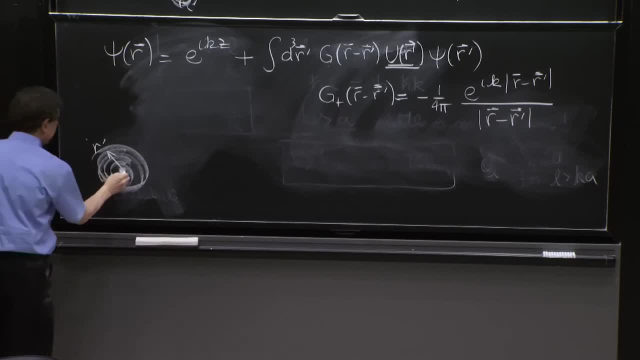 inside the range of the potential Here is 0.. And then there is an r, which is where you are looking at, And there is an angle between these two. Maybe I should make the angle a little bigger, Smaller, I mean. 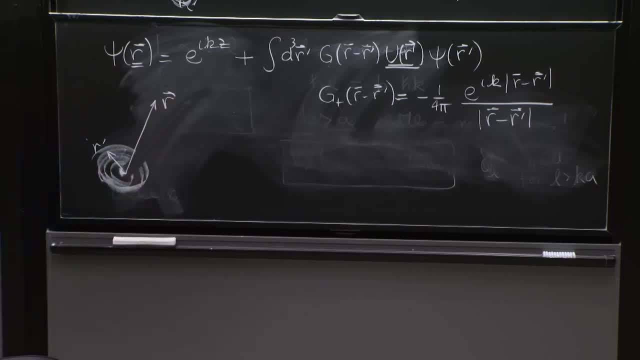 r And then, In general, we look always far enough. This is an exact solution, but we might as well consider looking at psi's that are located far from the potential. So we have the idea of what should we do with these terms. 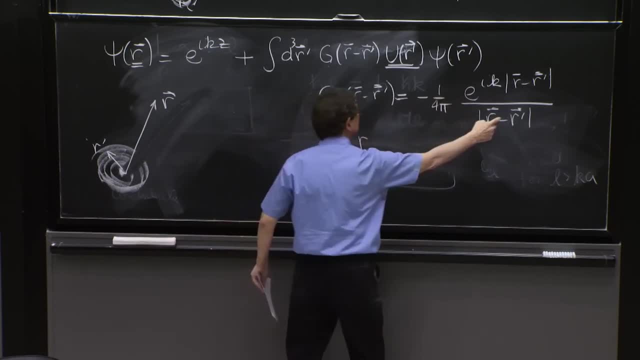 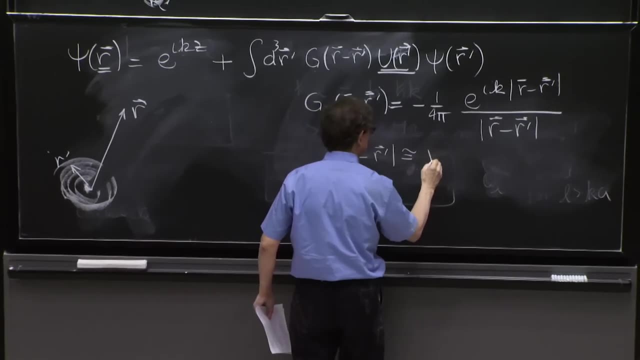 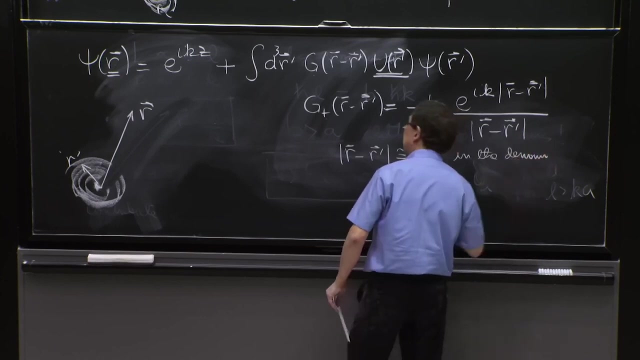 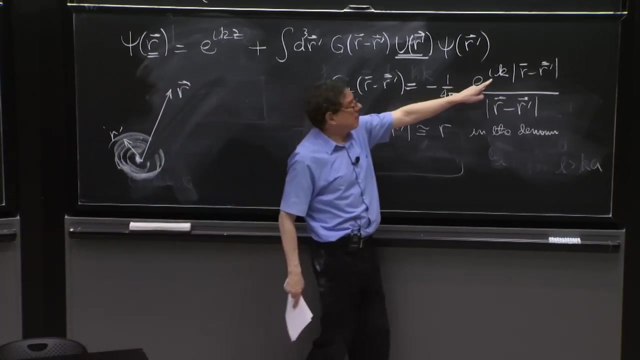 One thing you can do is to say that in the denominator here r minus r prime- It's good enough to set it to r in the denominator And for the numerator, however, it's a lot more sensitive Because you have a k here and depending. 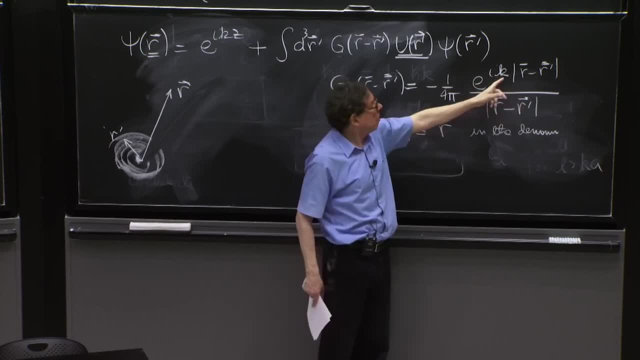 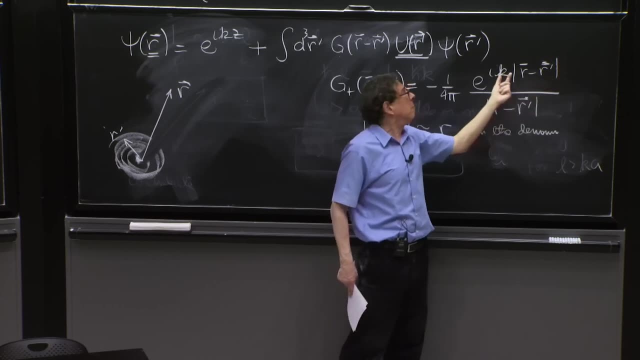 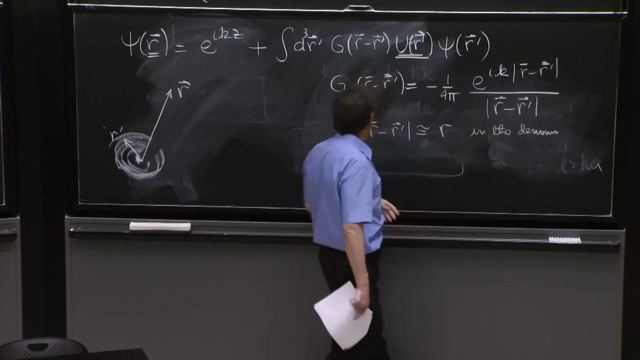 on whether k is large or small. a small difference in r minus r prime. if you're estimating this and you make an error- comparable, If it's comparable with the wavelength of your particle, you make a big mistake. If you're far away, you're 100 times farther. 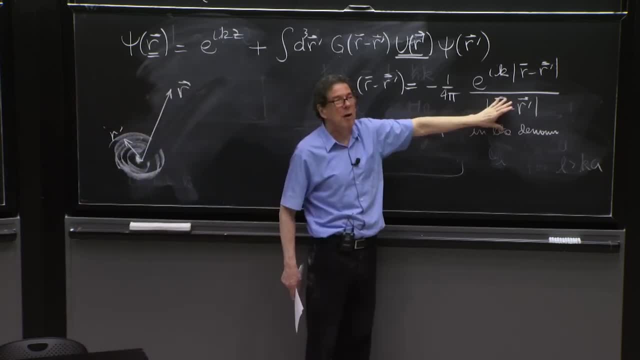 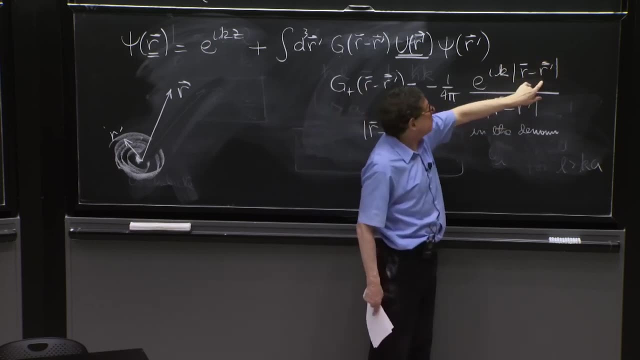 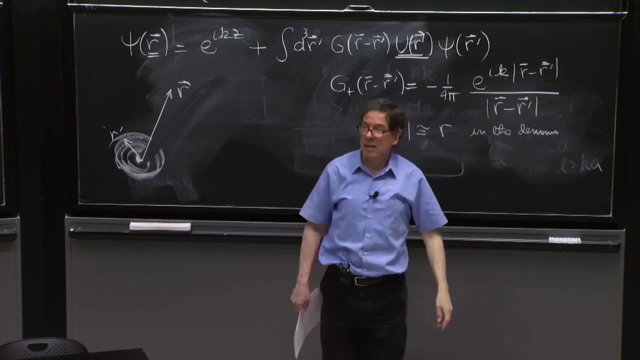 than the range of the potential. here you're making a 1% error, no problem. But if you're making a 1% error in the estimate of this, that may be still comparable to the wavelength of this k. So you have to be a lot more careful in the phase. 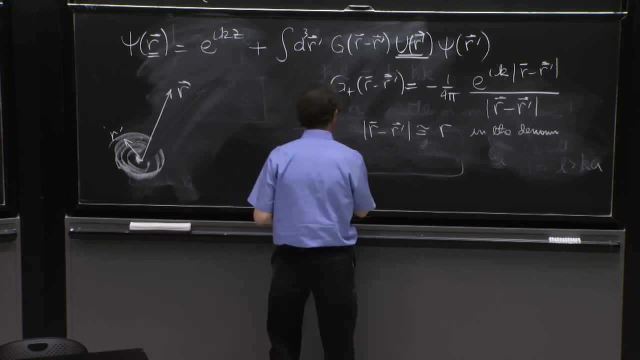 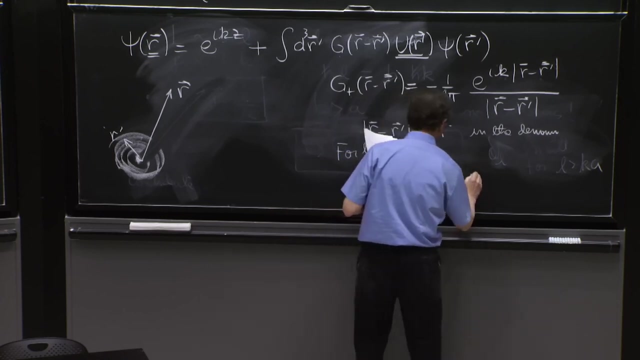 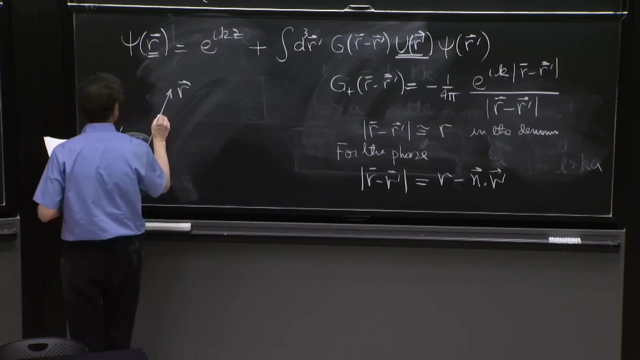 than you have to be on the other one. So, on the phase for the number for the phase, we will take r minus r prime, equal to r minus n r prime. So what is n? n is a unit vector in this direction. 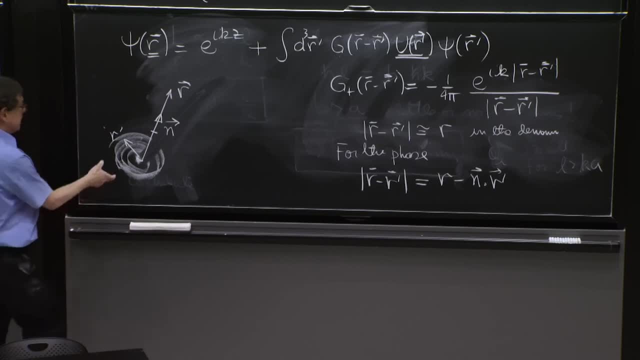 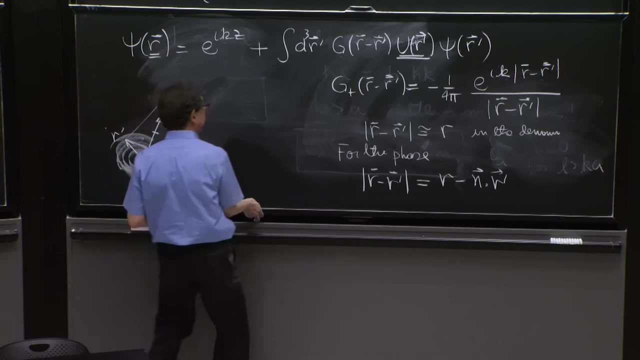 And indeed approximately this distance here is approximately equal to the distance r minus the projection of r prime into this one. So that is your approximate distance. So here is the final formula that we're going to write today. I'm running out of time. 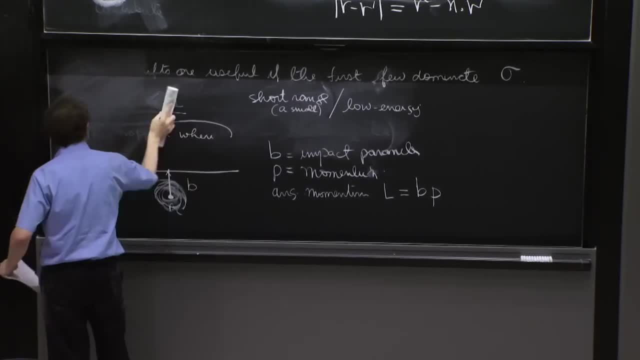 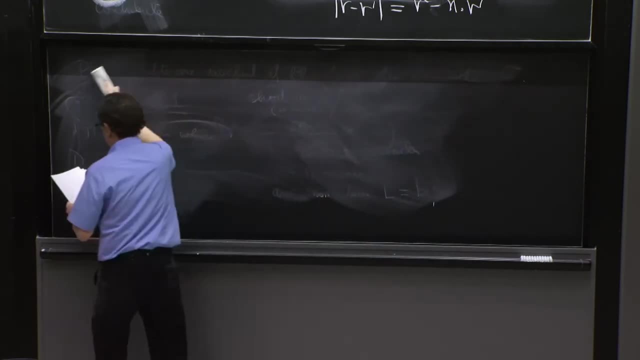 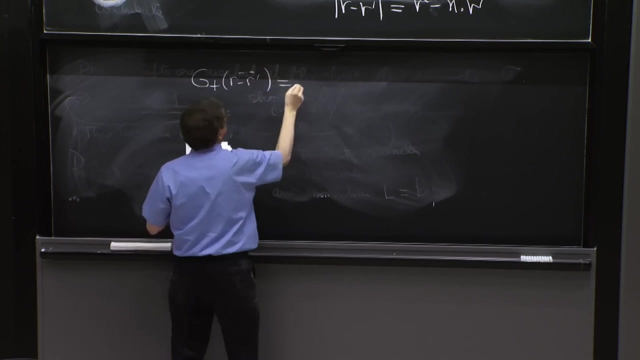 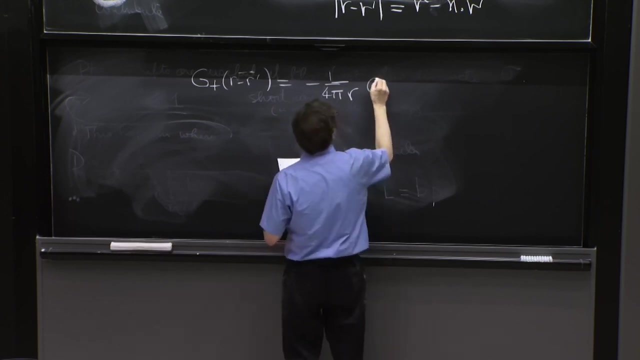 But that's it. That's what we wanted to end up with. So here is what we get. So g plus of r minus r prime has become minus 1 over 4 pi r. The denominator is r. There's an e to the ikr and then e to the minus ik. 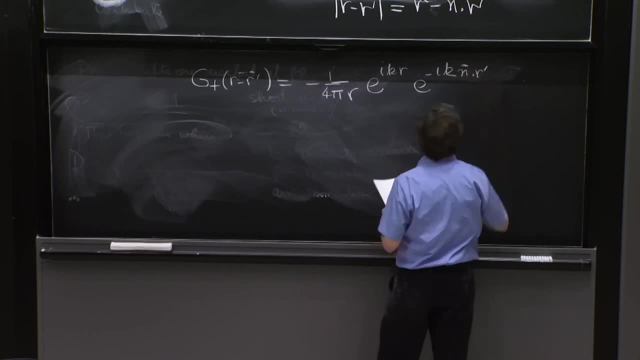 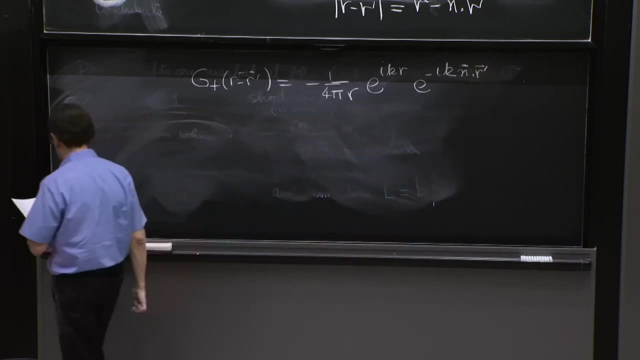 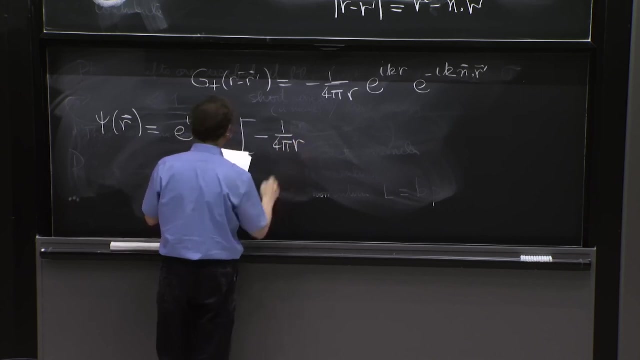 So this is minus 1 over 4 pi r, n dot r prime. So that's n dot r prime. So that's- and the arrows are crucial here. If I don't put an arrow somewhere, it probably means something. So psi of r is equal to e, to the ikz, plus minus 1 over 4 pi r.